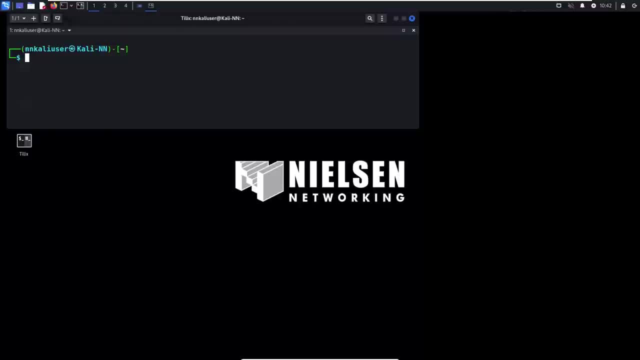 scanning tool. That said, this video will be focused specifically on Nmap when used for penetration testing. I give that disclaimer because we have other videos on the channel that offer a more generalized overview of Nmap and its uses, so that may be more your style, If so. 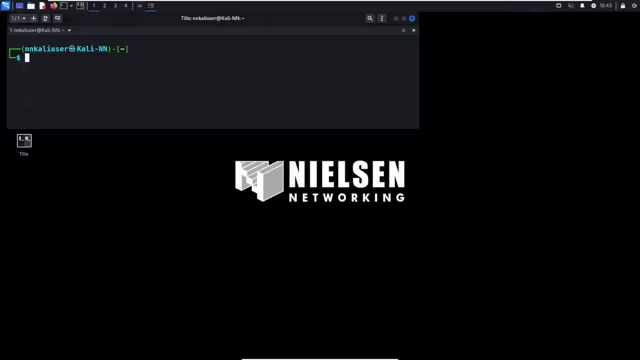 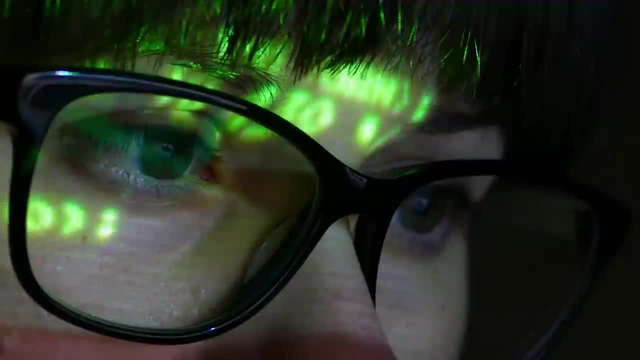 check out the link above or just go browse for it in the channel. Now, with that out of the way, and to reiterate, the focus of this video will be on Nmap from a pen tester's perspective. Now, what does that mean? That means I'm going to take you step by step through the 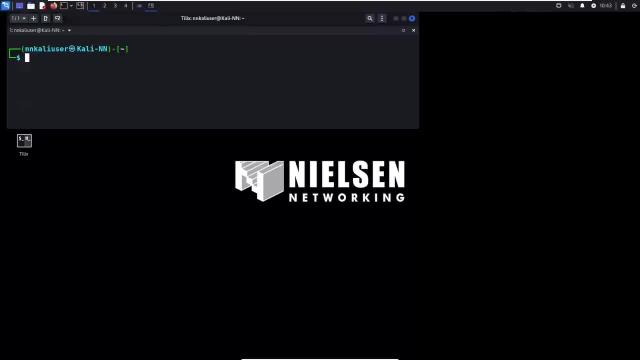 process of using Nmap for initial host discovery, all the way through vulnerability identification and exploitation, to show you why I believe Nmap is a must-have in any penetration tester's toolkit. So stick around as we explore the various functionalities of Nmap and learn how to. 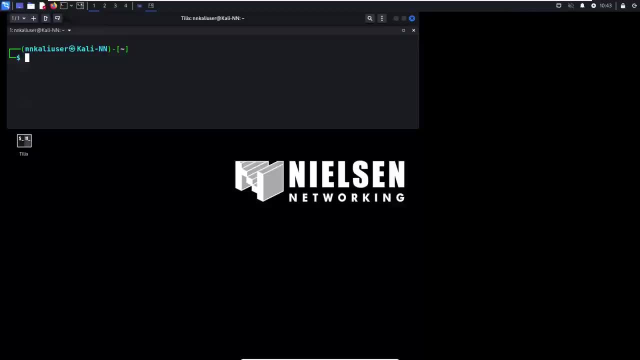 utilize them in your testing process. We're going to go from host discovery to advanced port scanning and service enumeration, and we're going to cover it all. Plus, I will show you how to use Nmap's advanced vulnerability testing features and how to take your results and use. 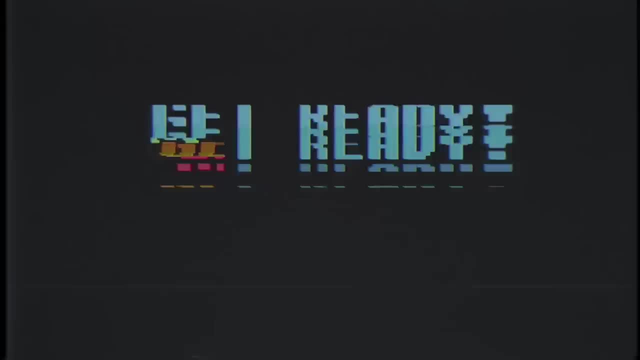 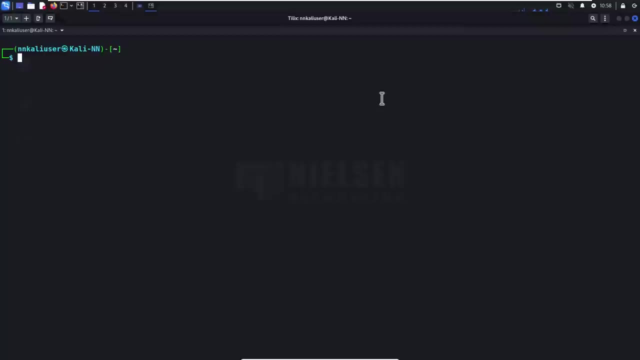 them with another tool to test any vulnerabilities that we do discover. So let's get to it. All right, and to get started here, I'm going to go ahead and maximize my terminal. I will be using Kali Linux for this video. That said, Nmap is available for almost every major Linux distribution. 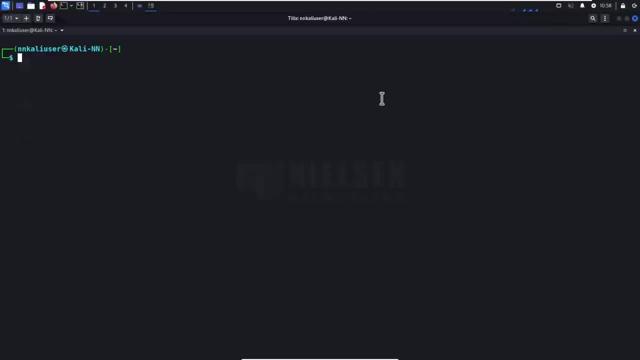 and even Windows. So that's that. I will be using this from the perspective of a pen tester. So remember that, And we're going to be sticking specifically to Nmap's uses in pen testing. I say that because we're not going to go out and do any open source intelligence gathering. 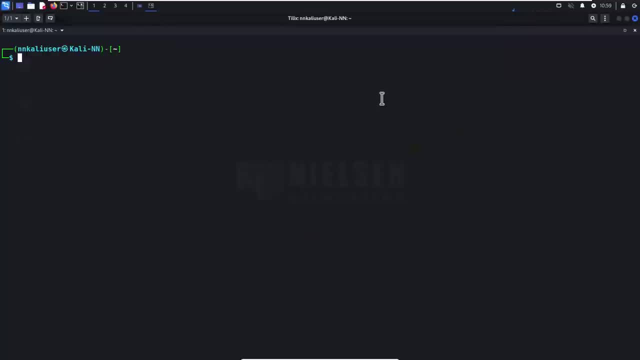 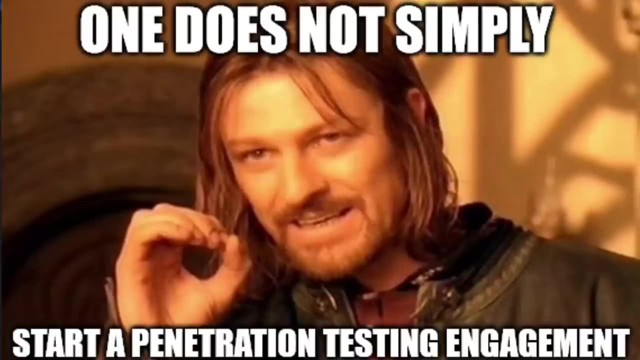 You know I already would have had permission from the network's owner that I'm performing these on. These are going to be performed in my own virtual network, So obviously I do have permission, But in the real world you would have needed, you know, to get the permission. 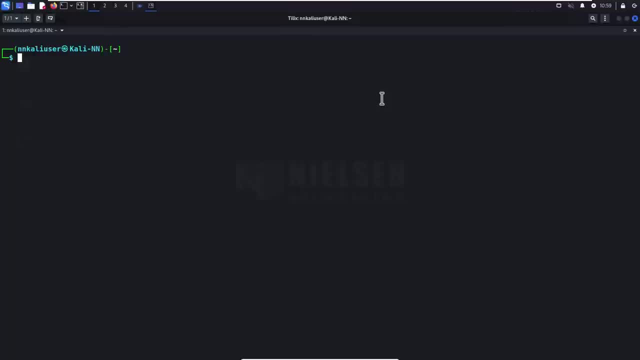 to get everything ready to where you're at the point. we are now on the network and we're going to perform this host discovery. So, that said, Let's get started with that. All right, And the first thing we need to do is verify the network. 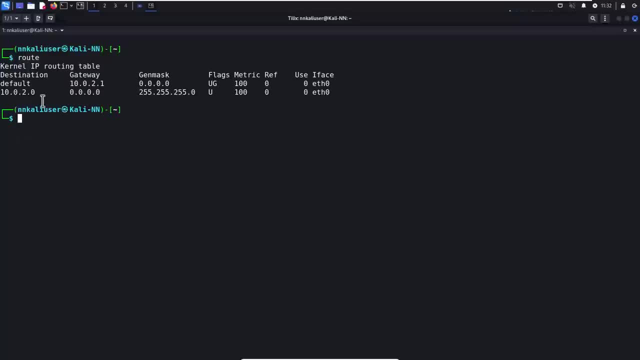 we're on. So we're going to type in route, hit enter And you can see right here: this is the network we're on And this is the default gateway. And to verify that we're on that network we can look at our IP address by doing an if config and verifying right here that that is the network we're. 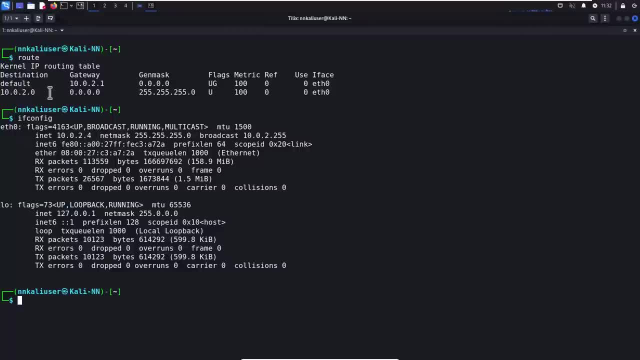 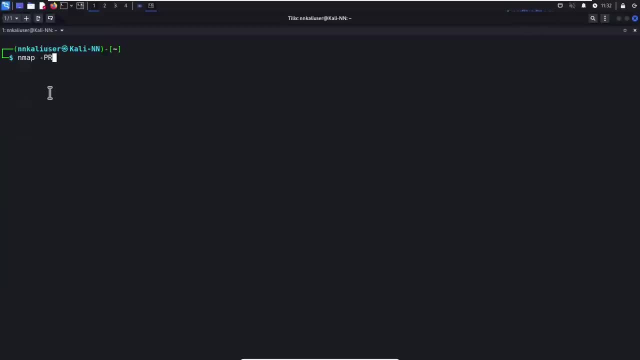 on. So we are on the 10.0.2.0 network, Good enough, And we're going to start off using this scan, And I'll explain what this is as soon as I'm done typing it. And just an FYI, all these commands. 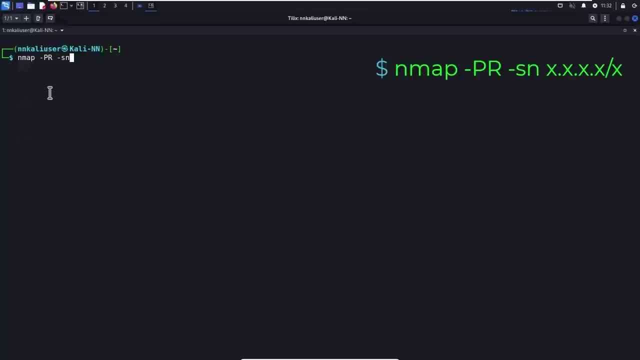 you'll be shown today are case sensitive, meaning if you do an nmap lowercase pr, you're not going to get the results you want and you'll be mad at me. So let's not do that. So case sensitive, And we're going to type in our network slash 24.. You could also do a slash 8 if you wanted to. 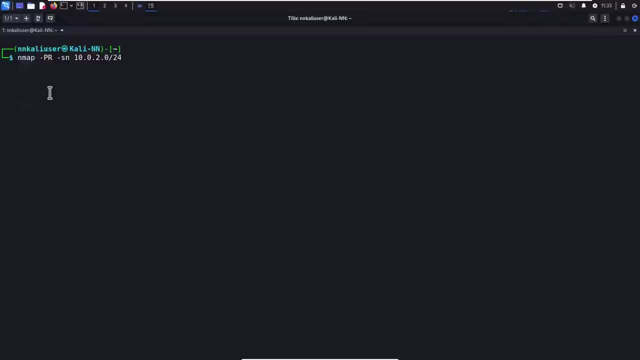 change the class of network you're scanning. I'm going to leave it here, because that's what I need for this, the purpose of this video. You could also write this this way if you wanted to, But it's simple. I think it's easier just to do a slash 24.. And then what we're going to do is: 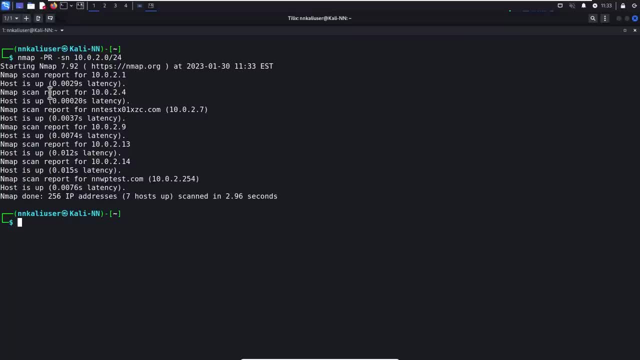 we're going to hit enter And we're going to let it do its thing, And while it's doing that, I'll explain what's happening. What this does is it goes out and it sends out an ARP broadcast request to each IP address in that range, So one through 254.. So, as you can see, it went through and scanned. 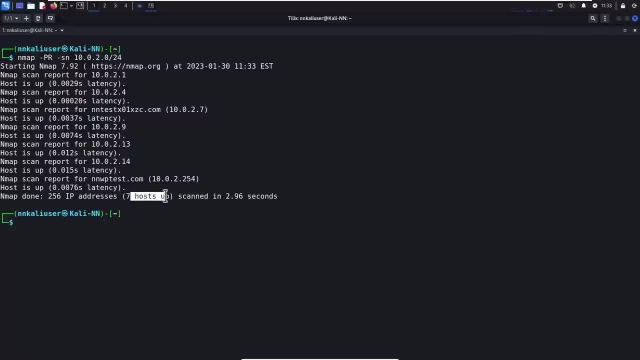 256 IP addresses and it found seven hosts that are up. The reason we do it this way is because we're trying to limit the transmission To only necessary transmissions. We don't want to go out and do a full-blown, you know. 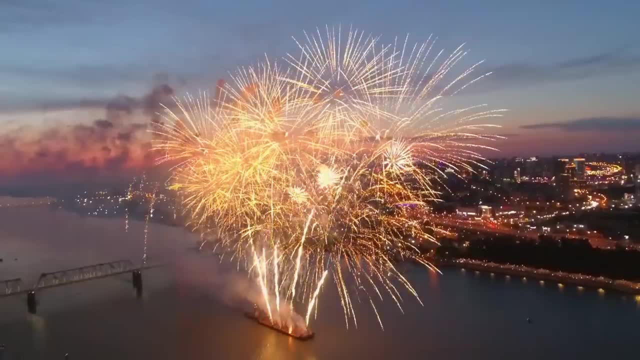 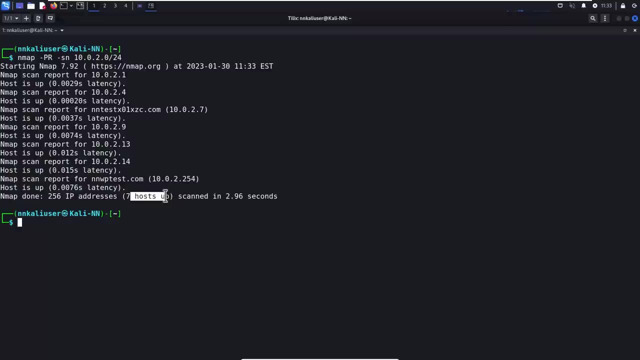 TCP discovery. Like we don't want to do that because that's like shooting a fireworks and going: oh, we're here. So we're going to start off as low pro as we can to get the information of the hosts that are available. We will then take this further, obviously, but we don't need 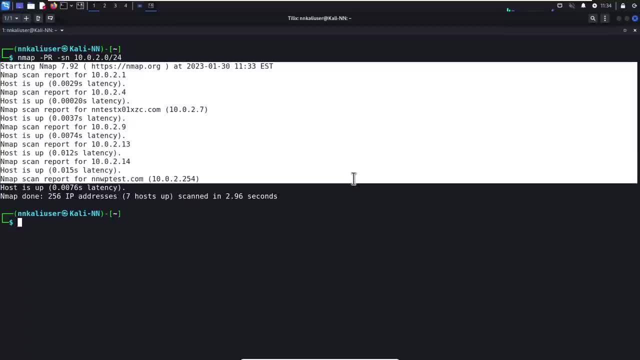 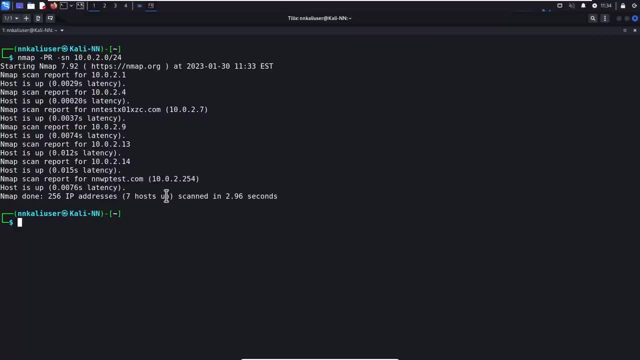 to then broadcast to the whole entire subnet because we know these are the only hosts on the subnet. So why do we need to send out a scan that scans 256 when there's only seven hosts? So now we can narrow down our search. Hope that makes sense to you. Now that we have the IPs we need, I'm going to go ahead and open up a. 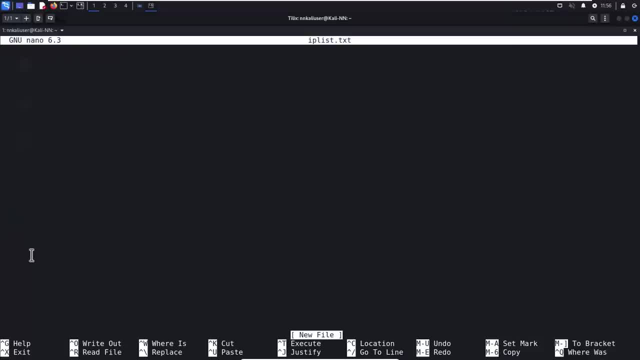 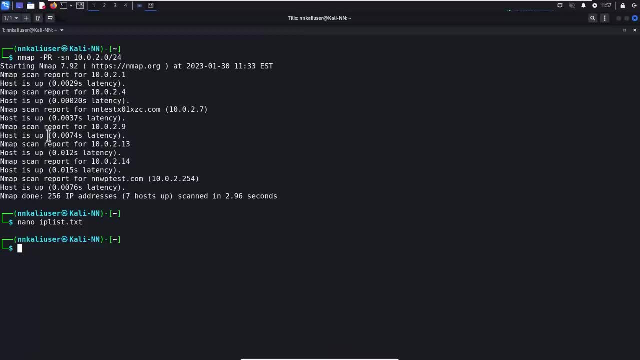 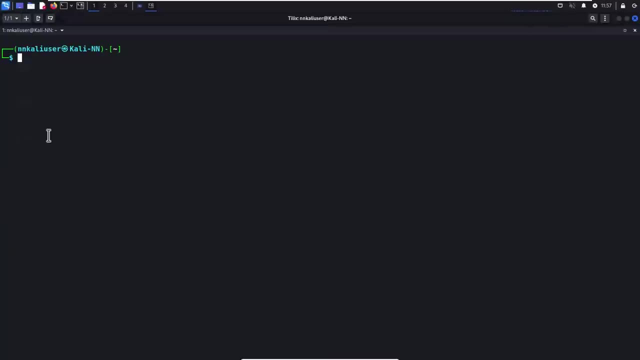 file here and I'm just going to call it IP list- dot text, And I am going to add the IP addresses that we just discovered. And here we are. I'm going to go ahead and save it and get out of it. Now that we have that, we are good to go. We no longer need to do network discovery on this. 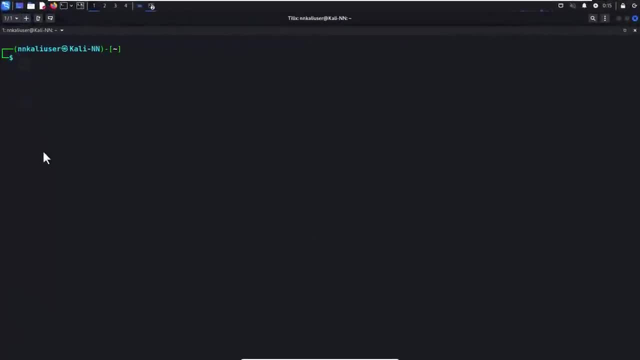 network. But what if you needed to scan an external website or an external network? You're going to need to use something besides layer two. So for that we're going to use a layer three scan, And here's how we're going to do it. We're 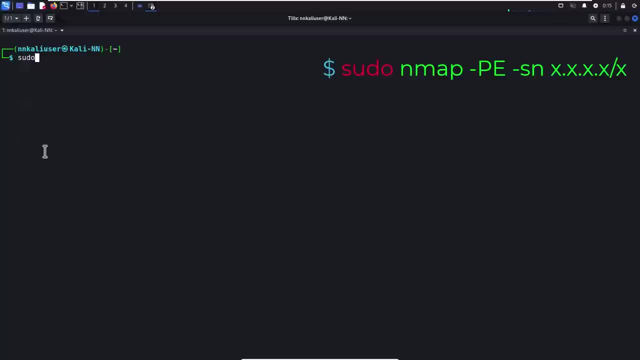 going to first use sudo, if I selected the active screen, And we're going to do a dash p? e, dash s? n And I'm going to scan a website that is actually hosted by Nmap. This is a free site. they put up that. they allow the general public to go and run Nmap scans against it So you can practice your. 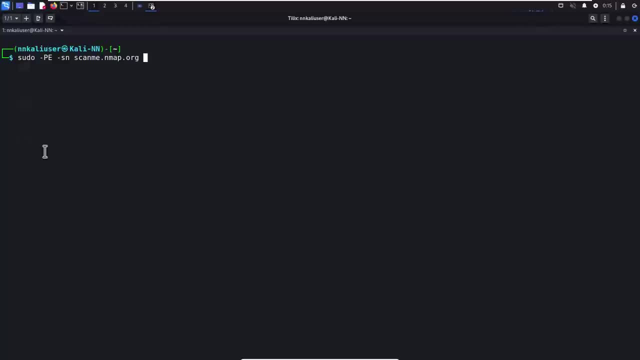 techniques on this website. Pretty cool that they do that. So we're going to go ahead and run this, And I guess I should put in the actual command, because that wouldn't have worked. So we're going to go ahead and do that And we're going to go ahead and. 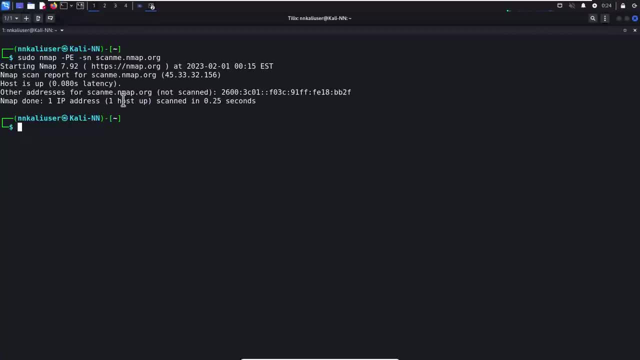 hit enter And our results came in really quick And it's looking like: okay, we the scan went through successfully. we know there is a host there, We know the IP is this And that is all we cared about. We wanted to verify that there was a host there using layer three, And we did, And 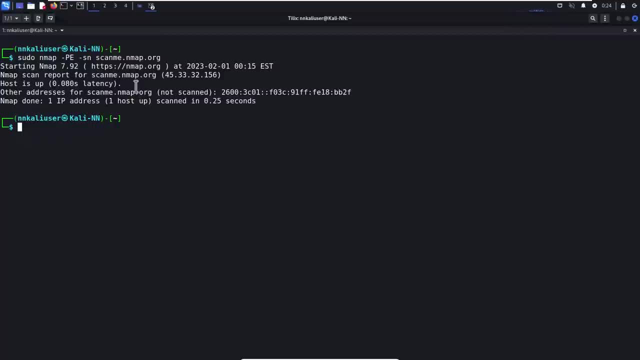 since we didn't use ARP, you may be curious about what we used. And we actually sent an ICMP echo request out there And that came back and let us know that there was a device out there. Now, if we would have done this against a bigger network, it would have taken a lot longer, because ARP is 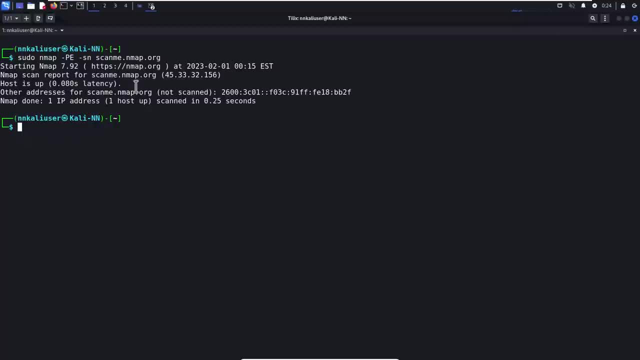 really quick compared to these ICMP echo requests. So just an FYI: if you're going out there and you are doing this against a bigger network and it's not returning as quickly as you would expect, that's why it's totally expected behavior. So that's that. Now let's say that didn't work. The 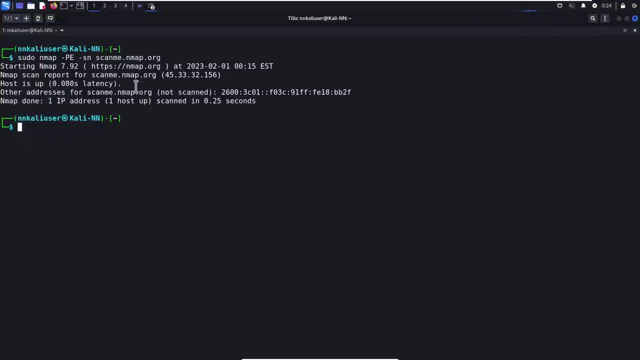 reason likely is going to be because the firewall is in your way And it's saying no, no, no, I'm blocking those requests. So you're like: dang it. what do I do now? Well, now we're going to go and 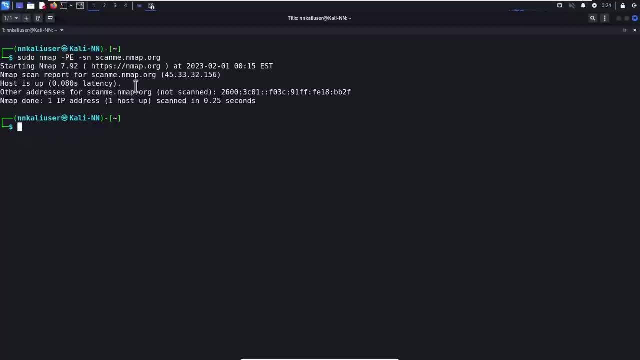 try layer four. And how we would try layer four is as follows: First thing, we'll clean this up, And then we're going to want to go and map dash PA 80, report 80. And we're going to do that again And we're 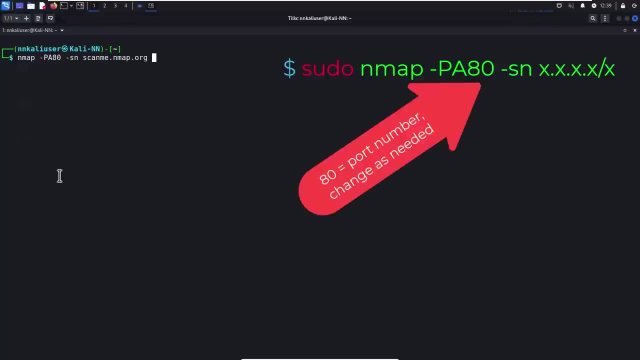 going to do scanmenmaporg once again And we're going to hit enter And we got what looks like the same results as the layer three, And it is the same results. I mean, it's not warning us about using ICMP, that we need root. 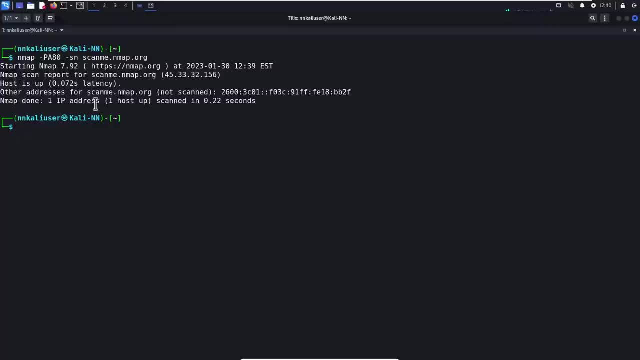 But nevertheless, we got the same. we got the IP address and we got that. it is up Now. it doesn't look a lot different to you, but it is, And what's happening is we're actually using layer four. we. 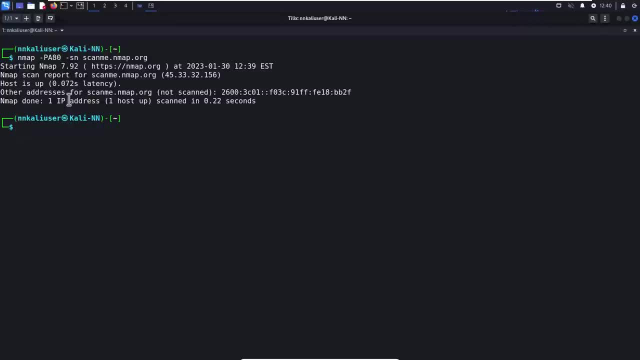 sent acknowledgement packets to the host And, as a result, the live hosts responded with a TCP RST reset packet indicating that we have received the packet and there is no open communication channel. That means the host is up. So if this were a firewall, this would have gone through and 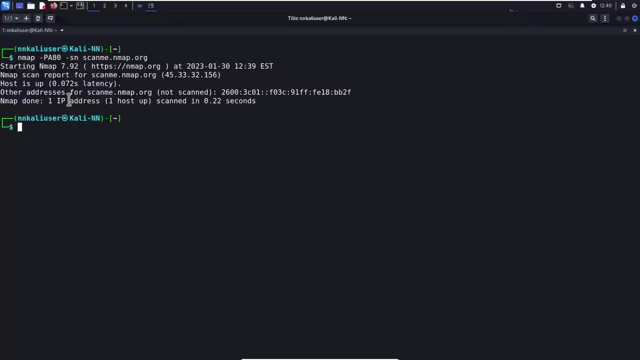 showed us that the host is up on this IP range, And that's what we wanted to accomplish. So now that we know how to do that, we're going to go back to what we discovered in our layer two scanning using ARP, which is my internal network, using my internal devices. So let's get started on those. 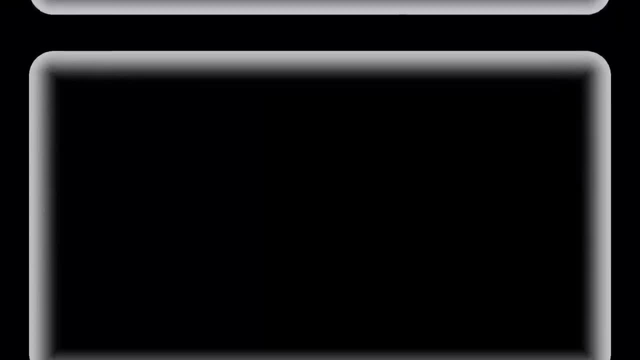 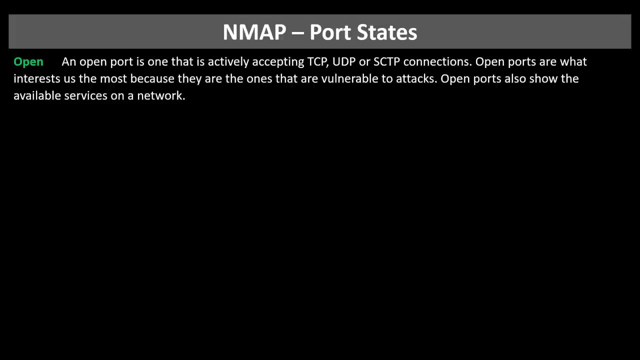 I'm going to go ahead and clean this up And we'll get to it All right And real quick. before we get to port scanning, we need to understand what we're going to be looking for And specifically, we're going to be looking for the port state we want to see. 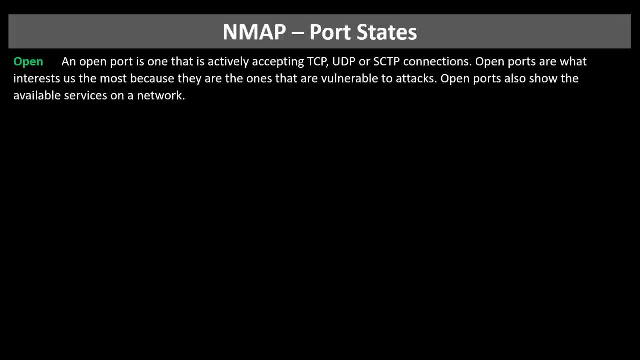 the results come back that the port is open. This is good. good this means that it's accepting connections, whether it's tcp, udp or sctp, obviously we're going to be looking for the first two. if it comes back as closed, not good. that means it's closed and 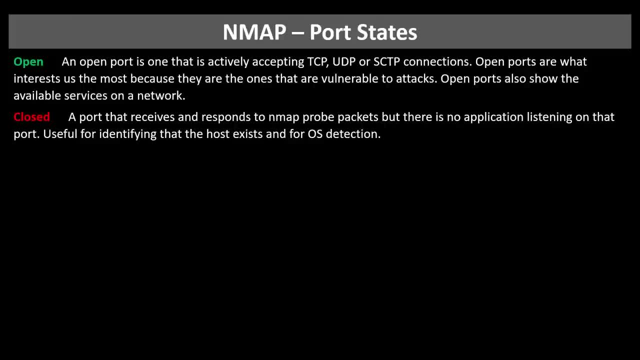 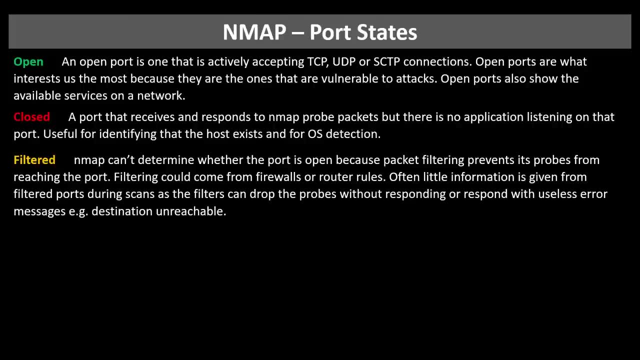 other than verifying that there is a device at that ip address. there's not much else we're going to be able to do at this point with nmap filtered. this is a very vague response. doesn't help us out that much. i'm not going to waste time explaining it. feel free to screenshot this or pause the video. 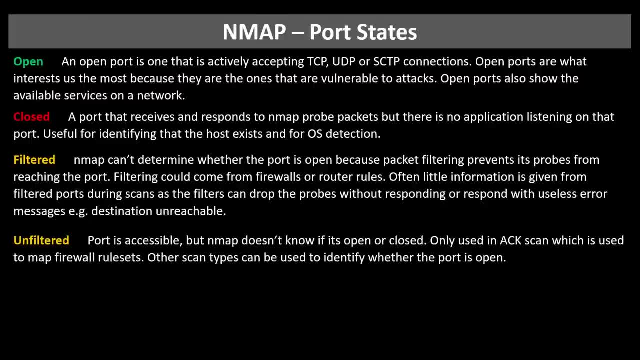 and check all these out with more detail. if you want unfiltered, this means it's accessible, but i can't tell if it's open or closed. not the most helpful, but it does suggest that you go and scan, maybe using a different technique. maybe you use a layer four or layer two or layer three, whatever. 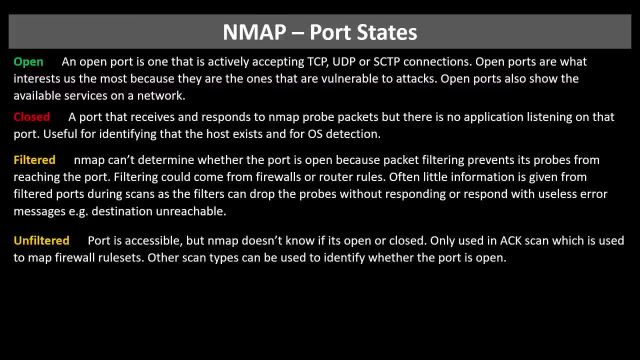 you initiated with. try a different method and see if you can get a little further open filtered: similar, but it's unable. nmap was unable to determine if the port was even active, so a little less useful than unfiltered. last one: closed. filtered pretty much means it's closed, so the 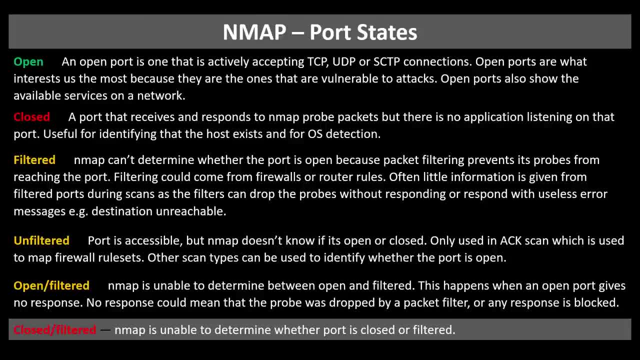 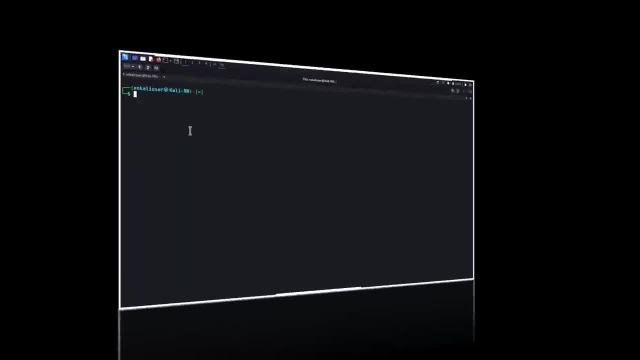 really the ones we're really going to look for are open and unfiltered. the other ones we're just kind of like, eh, not really worth the time. So, that said, now we're going to move into the port scanning. All right, we're going to start with the most basic of all, Nmap scans, And that. 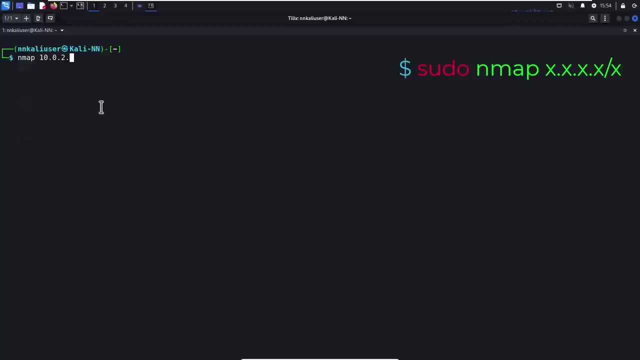 is going to be Nmap, and then the IP address of the device you want to scan, Hit enter and boom, just like that, your first scan is done. Now, what did this do? This scan scans the first thousand most commonly used TCP ports and then returns the results. So it scanned them against. 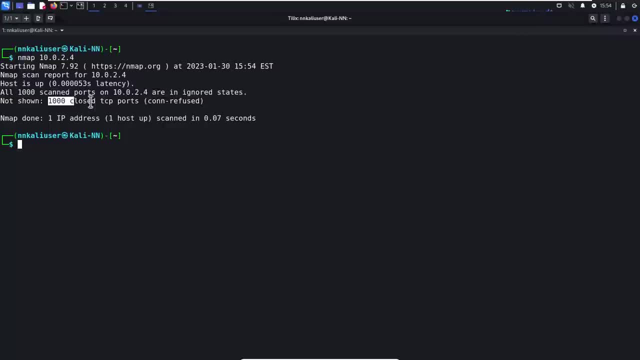 my Kali Linux box that I'm on right now and they all return that they are closed. That's good. I didn't expect them to be open, but that is how you could do it. Now let's say you wanted to do. 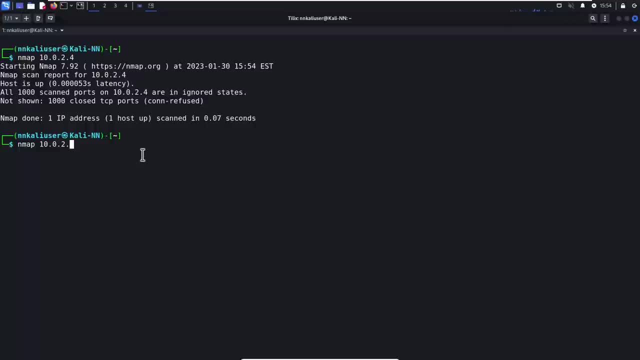 this to the entire network. You could do that, but instead of doing that, you would do this. But again, remember what we did in the beginning. We did host discovery so we could stay low, pro, under the radar. We don't want to, you know, shoot up fireworks again. We want to stay under. 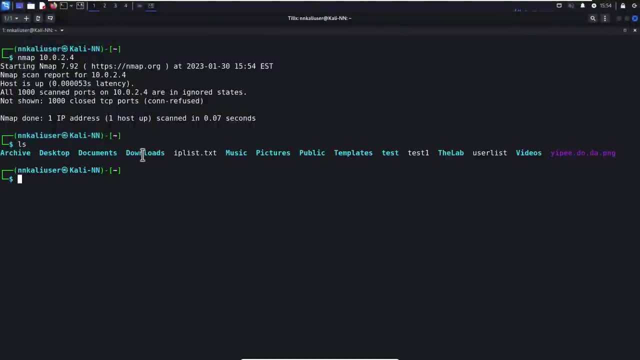 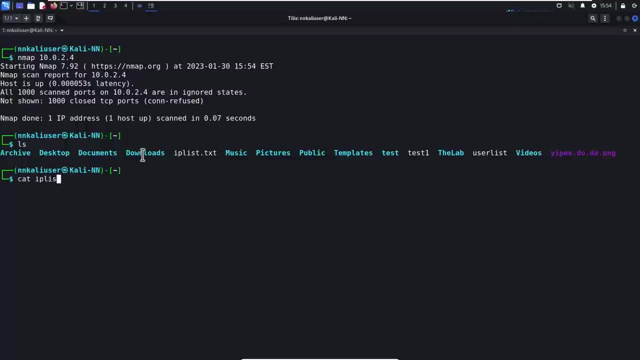 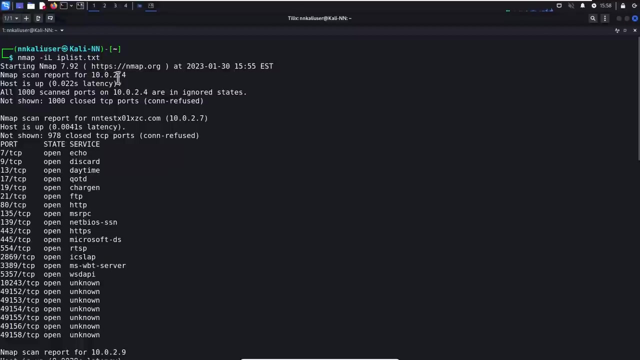 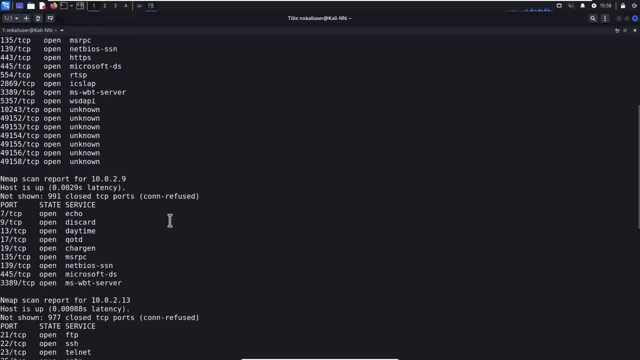 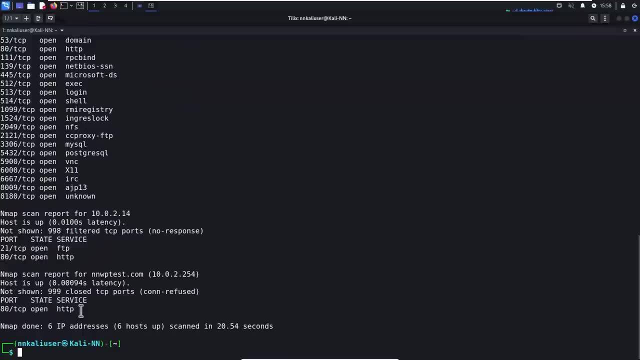 like it has a lot of stuff we'll look into further. I keep continuing down here. 2.9 has some stuff we'll look into. 2.13,, 14, and 254 has at least port 80. So all the other devices look to have. 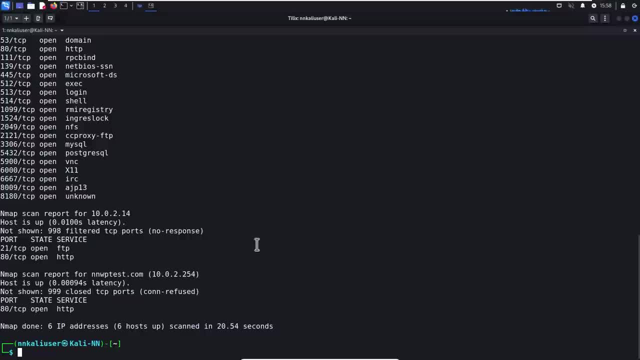 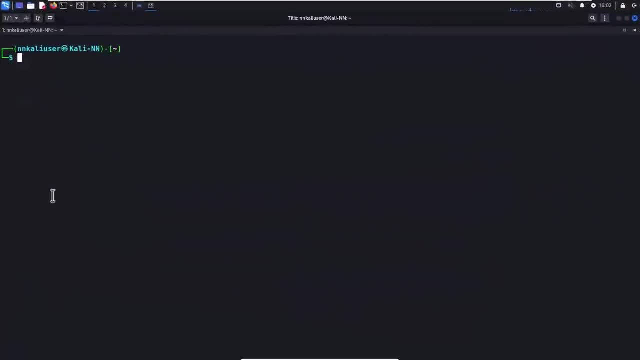 something we can investigate a little bit further. So let's go ahead and move on to the next scan we could look into. All right, This next scan is going to be useful if you are looking for specific ports. So let's say we were. 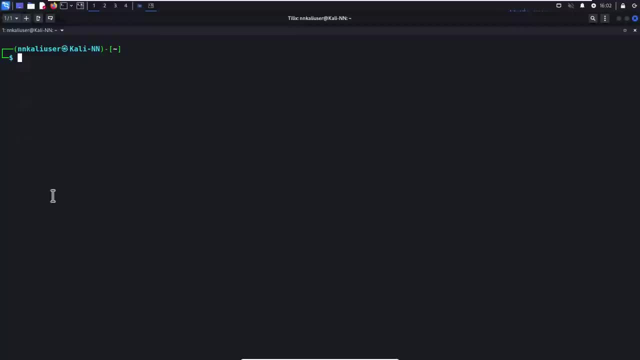 looking to see what devices had SSH open. So what you would do is you would go in map, you would do a dash P and then you would put in: what port are we looking for? Let's say 22.. So then we would put: 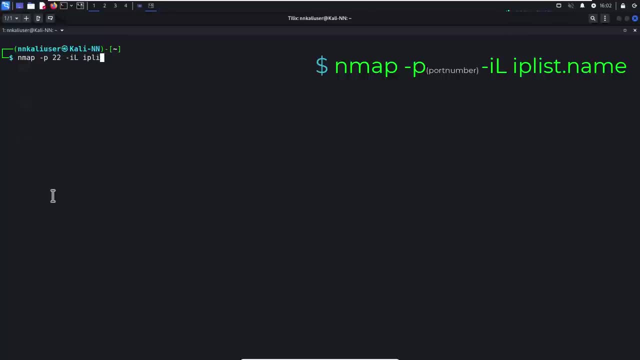 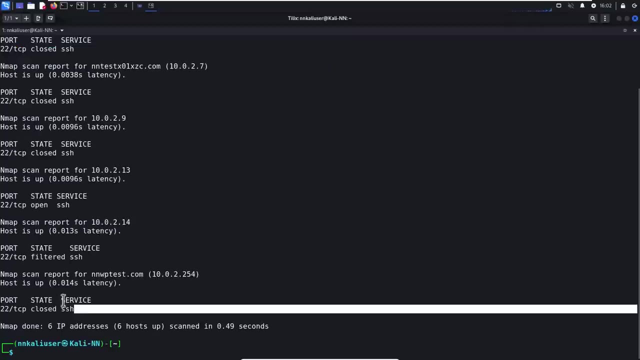 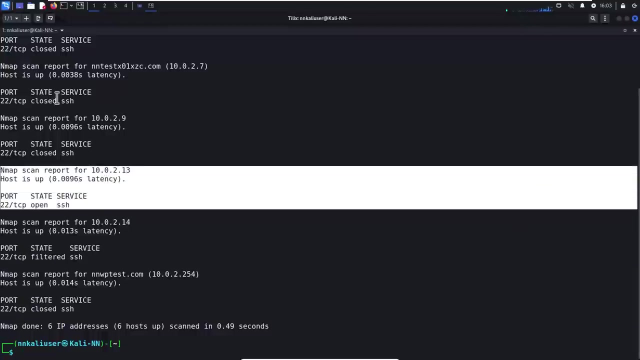 in dash IL to point to our IP list, and we would put IP list dot text, Hit enter and wait for the next scan. It's filtered here, It's open here. So 2.13 is open, Closed, closed, closed and it looks. 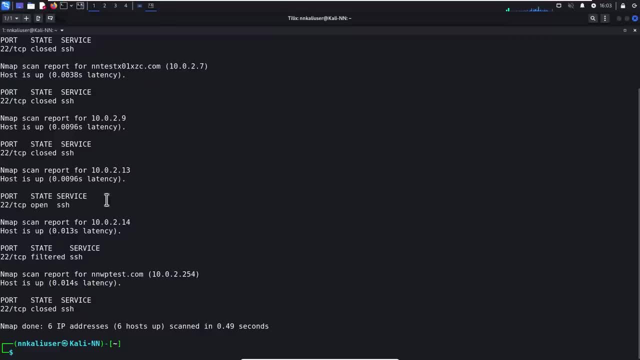 like it's closed on all the other IP addresses, But we do know now we could investigate SSH on this one. So see that can be useful. Let's say you wanted to do the same thing but you wanted to do it for port. let's say 80. See how many of them are running web servers. You can see right away. 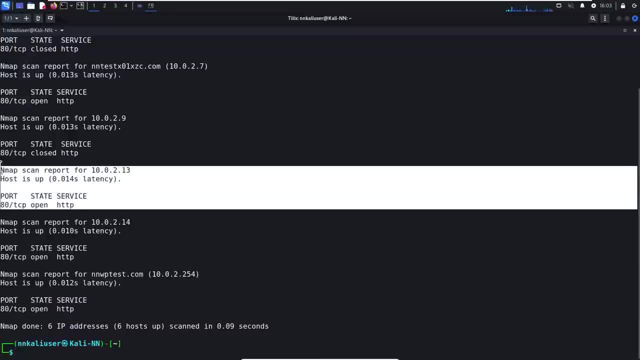 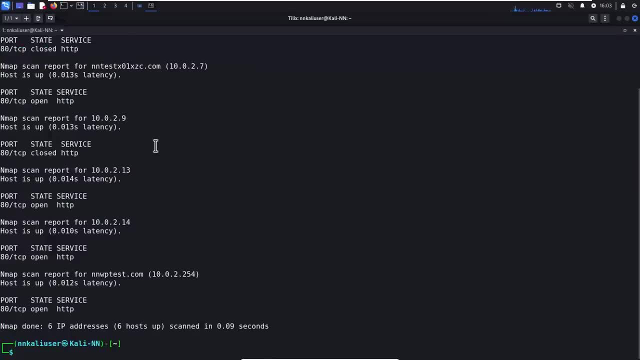 That's unbelievable. So right there, port 80 is almost open on all of them. So you can see how you can do that and you could even combine it. Let's say you wanted to do 80, and you wanted to do let's just say 21.. Let's see, And it would go through and you could combine them. So you 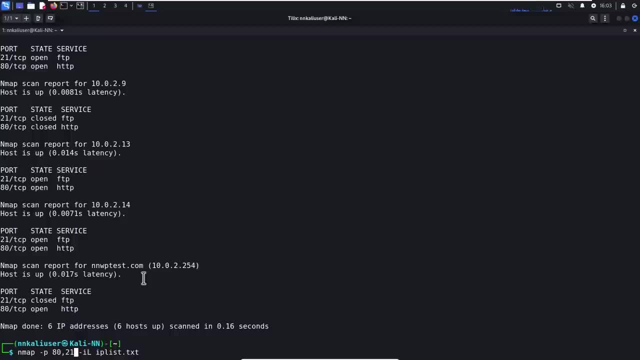 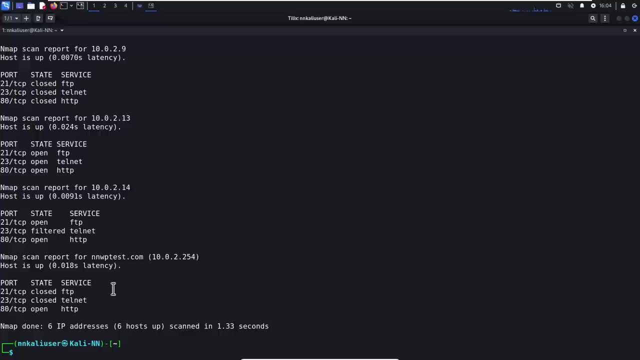 could continue to chain these along. Let's say you also wanted to know if 23 were open, You'd have to wait a little bit. longer you put, the longer it's going to take you to get the results. obviously because it's doing more. 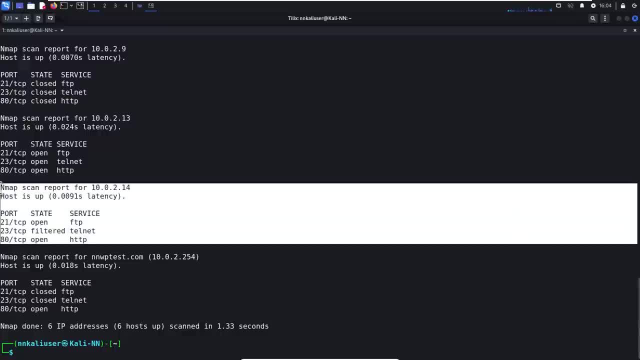 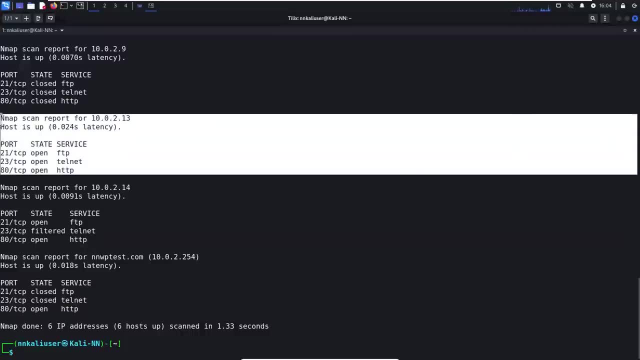 makes sense, right? so you go through here and look at this: this one has ftp is open and http is open. let's see if any of them- oh, look at this guy right here- all three are open. so that would be a prime target. so, that said, that is how you run with a specific or specific port. all right, we're going. 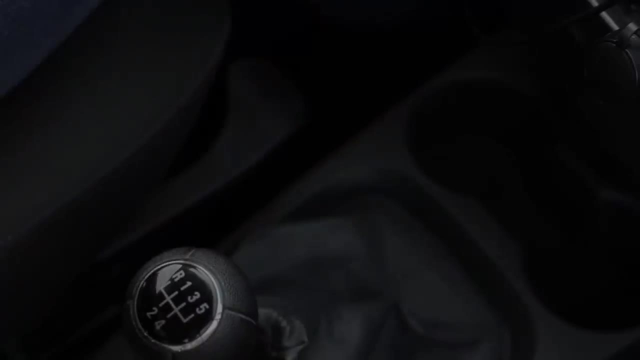 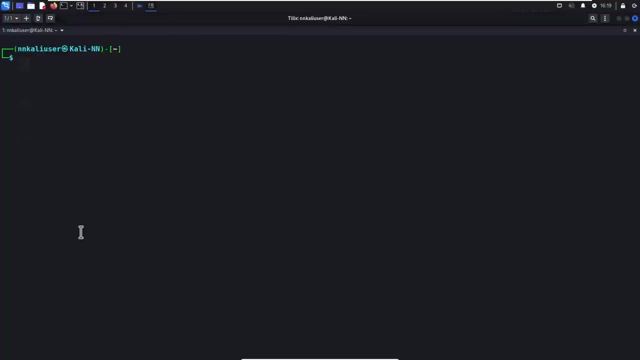 to shift gears here a little bit and we're going to go out and we're going to scan for filtered ports. and i know you're thinking: well, why would we want filtered ports? we want filtered ports because we're looking to see if the ports happen to be there and they're just being blocked by. 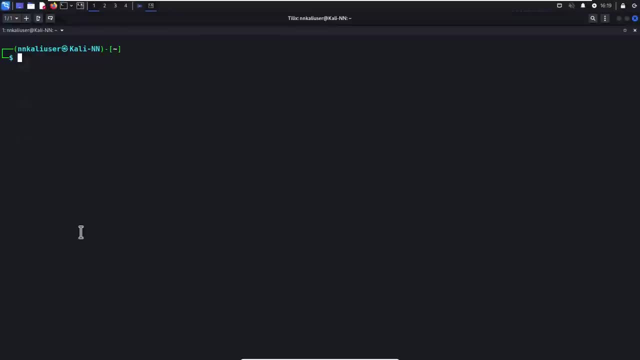 firewalls or other devices, and by looking for these filtered devices we'll know other ports we want to investigate further using different scanning techniques. so to look for these filtered ports, we're going to go ahead and do the following: we're going to do nmap as normal and we're going 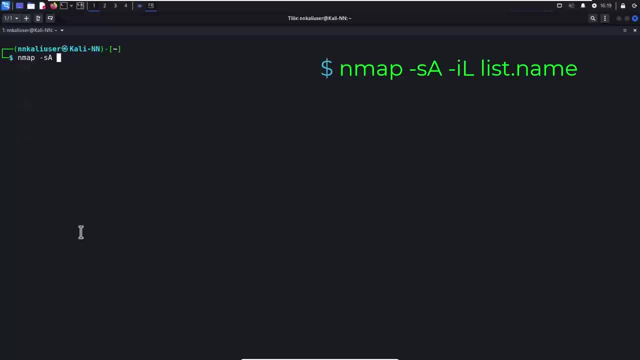 to do a dash s and an uppercase a, and then i'm going to tell it to use my ip list. again, you could tell it to use a specific ip or a range, all that good stuff, and i'm just going to stick with this. we're going to go ahead and run it and it's going to warn you you need root. so what you're going to. 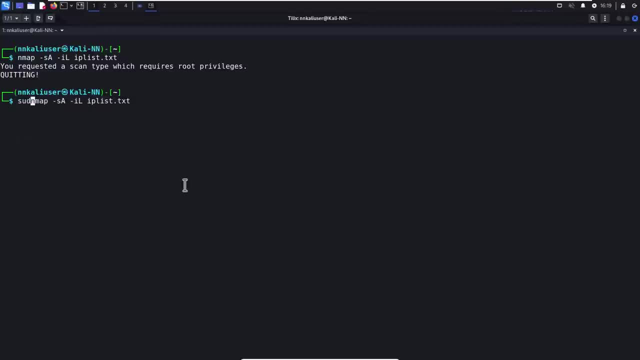 need to do is either you know su to root or use sudo. oops, you're not going to use su because or said said, so it's not going to work. we need sudo. so we're going to go ahead and hit enter and let it do its thing. all right, and the results are in. let's take a quick look here. uh, we'll go from the. 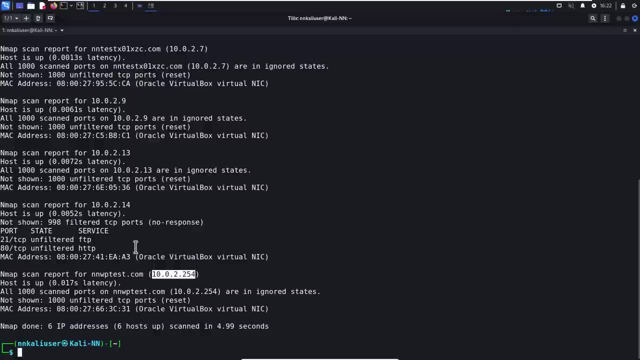 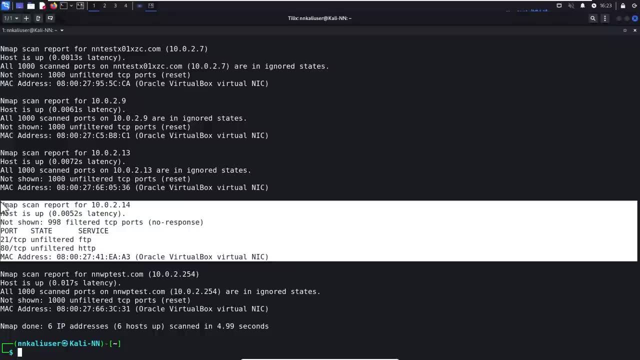 bottom up this time, so it's looking like 254 is not having anything but right here. look at this. these are showing as unfiltered, and remember unfiltered doesn't mean that it's open, but it means it's accessible. so that means we'd want to. 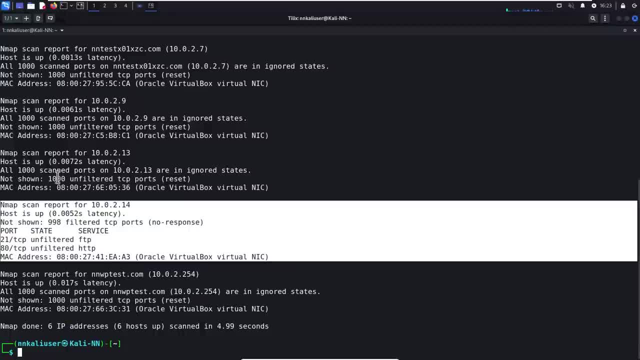 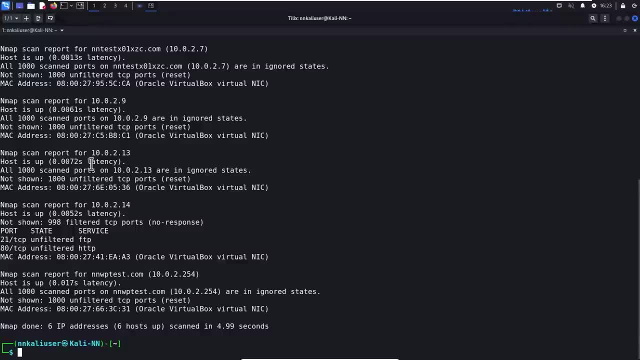 further investigate that and see if we could get in on port 21 and 80. so let's continue up. none here, none here. so it looks like everything else reported as either it was either showed open in another scan or it's closed. so this would be the only server we'd want to further investigate on. 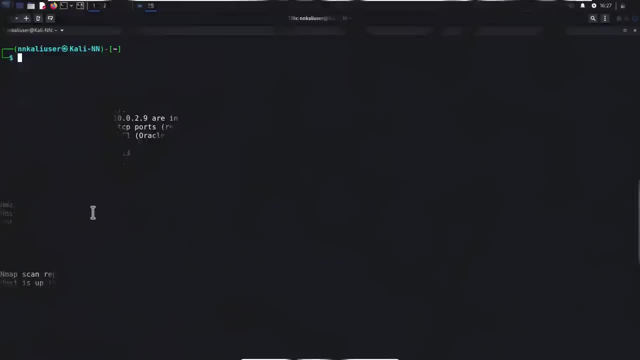 port 21 and 80. okay, let's try something else here. all right, i think it's about time we look at some udp ports, because we have completely overlooked those until now. and, believe it or not, that happens more than you would believe, but you're not going to. 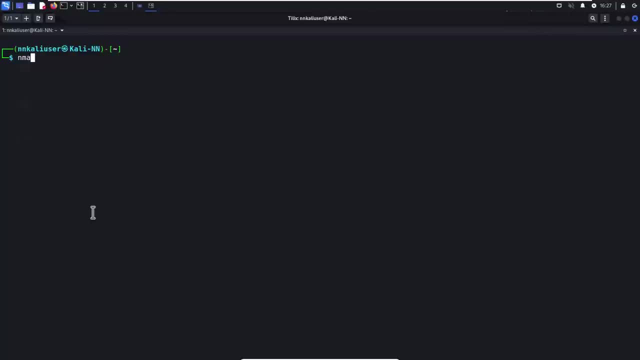 let that happen, because you're going to be thorough and to do this, we're going to go with an nmap, like we do with all our commands, and we're- for we're going to go sudo and map, i should have said- and we are then going to put in a dash s and a u for udp, and then we're going to go ahead and put in our 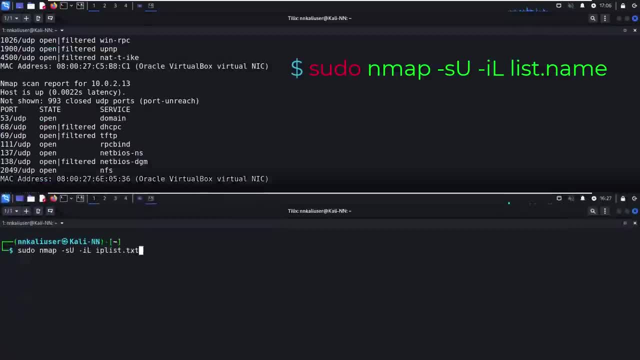 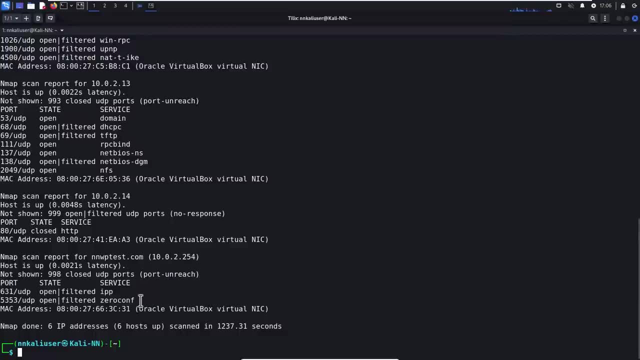 file for our ip list and we're going to let it run. all right, the results are in. let's go ahead and take a look here. so it looks like it's just a little bit different from what we saw previously. um, it looks like this first server is showing us that it has some open slash filtered, so that's not going to be super. 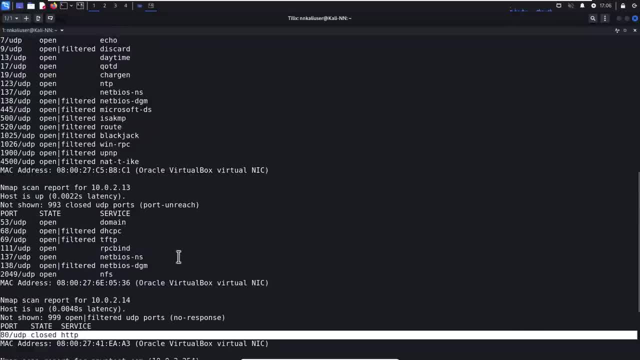 useful, so we won't spend too much time looking at that. this is showing that it has a closed udp port, so that's not super helpful. um, i'm assuming tcp is open on port 80.. that's why it's showing us that, and then this has a combination of it. looks like dns right here is open, so that's something. 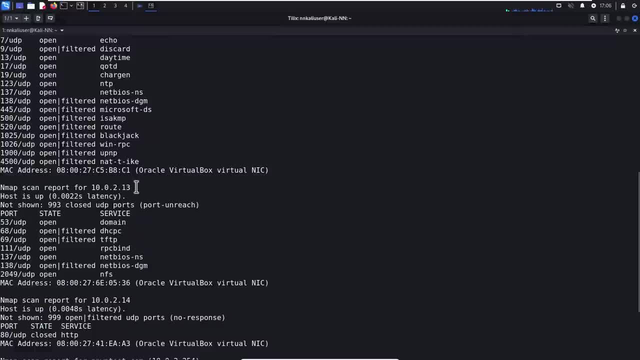 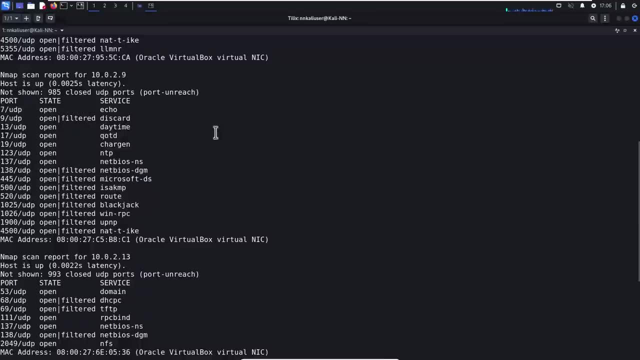 we would look into. and then it has some open, filtered, and just some more open. so that's 2.13 and moving up the ladder here we have more and more open on the next machine up and it just kind of keeps going with more and more open all the way up. so you can see scanning for udp was. 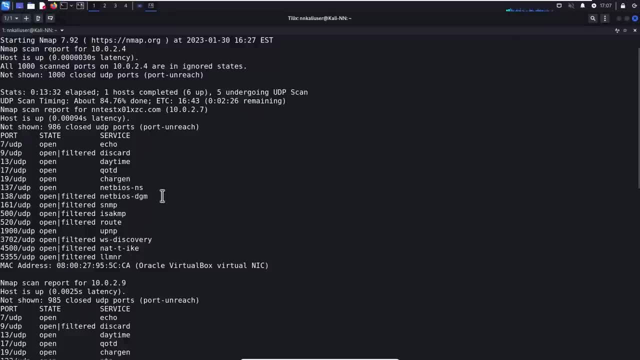 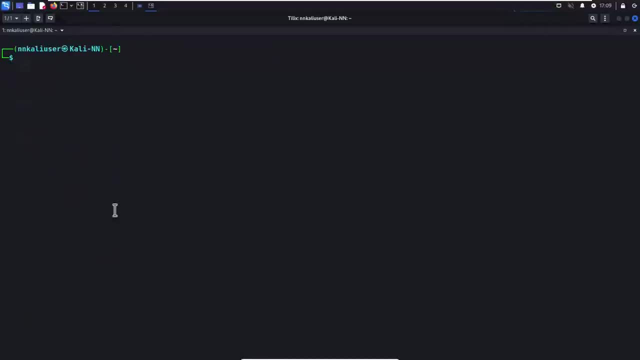 definitely useful, because if we didn't do this scan, we would have been in the dark about some of these other ports that are open that we could have investigated. so let's go ahead and check something else out. all right, for the next step. we want to take this a little bit further now. we've 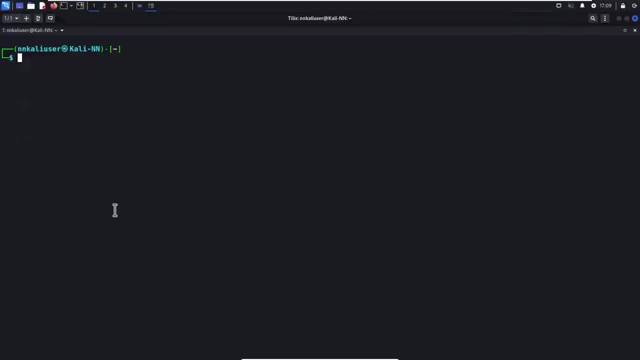 found some open ports, both udp and tcp, but now we want to know exactly what services and version are running on those ports. so to do this, we need to switch it up a little bit and we're going to need to go with nmap again. we're going to go sudo just in case we need it, and we are going to do a. 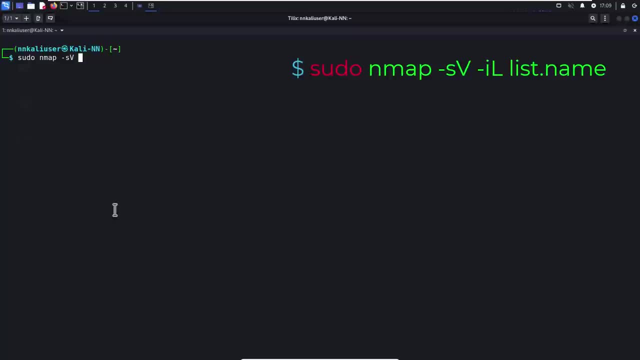 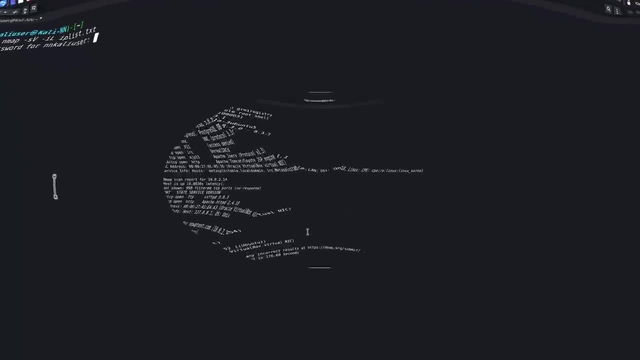 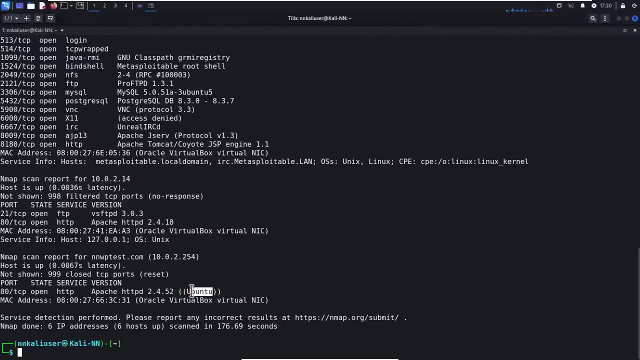 wait for the results here after i put in my password. all right, and the results are in, so let's take a look here. first thing we'll look at is 2.254, which apparently is a umuntu server, and we knew port 80 was open on it, but we didn't know what was on it, and apparently it's apache. 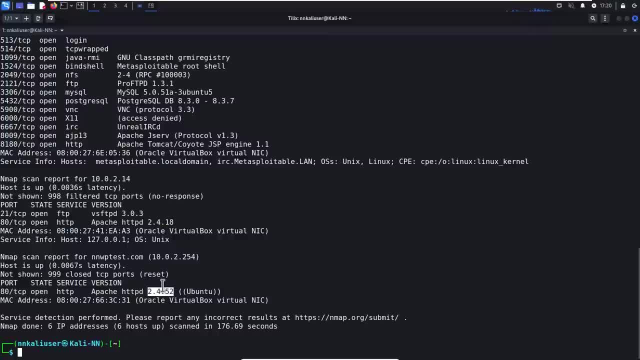 and it's running this version of apache, so you can see how powerful this is. now we could go out on google and just look up vulnerabilities for apache 2.4.52 on linux. going up the ladder, we could do the same thing. going up the ladder, we could do the same thing. 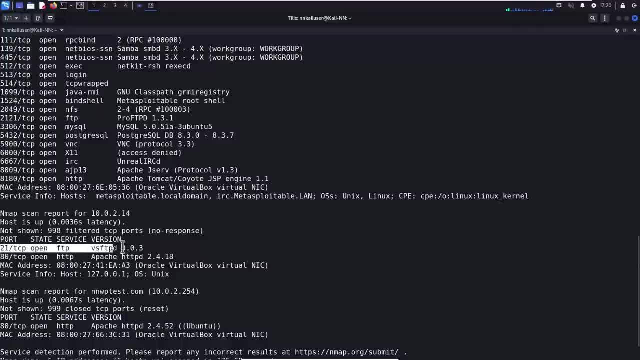 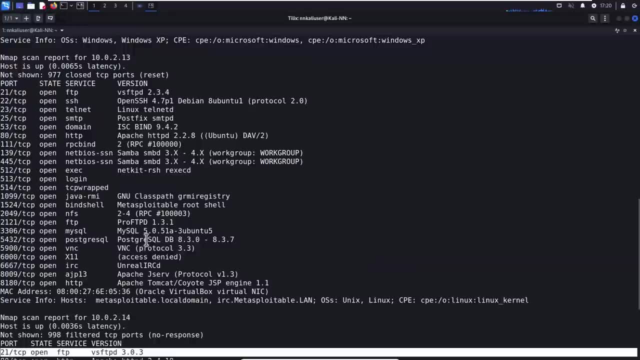 for the next server, but this one is also running an ftp version here, vsftp 3.0.3. so again we could go out and see if there's any vulnerabilities for that version of that ftp. and up here this thing has. you could almost just blind throw something at it and hit a target here. 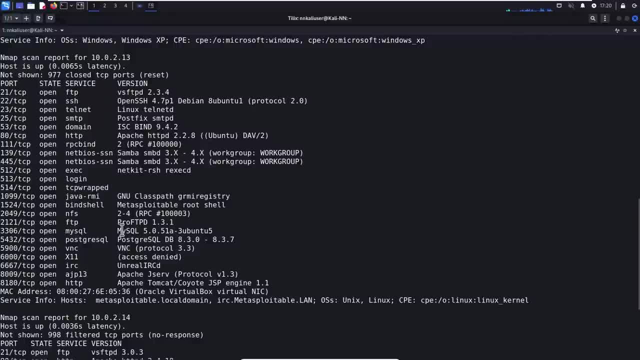 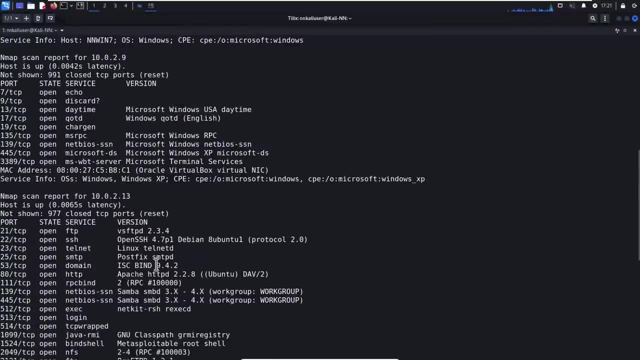 i mean this is a lot of real estate to deal with here. my sql, i mean ssh tell, i mean my gosh, there's a lot there, so that's definitely one. we would be, uh, targeting actually my sql, i mean sqlcom, which is a lot fancier than the vmware one. 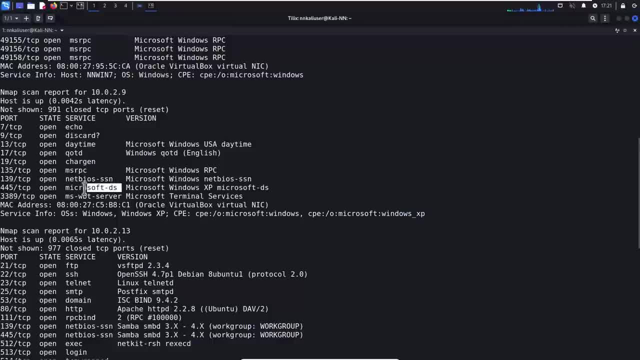 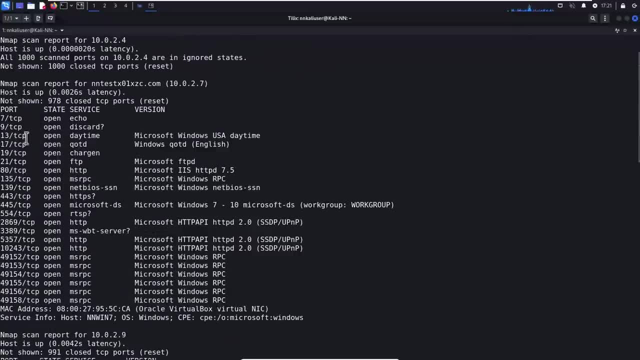 and this is actually going up the ladder again. we have another machine on 2.9 that looks like it has a few things. looks like it's running um smb and some other things here, so that's another one we'd look into further and continuing up. look at this: this has a. 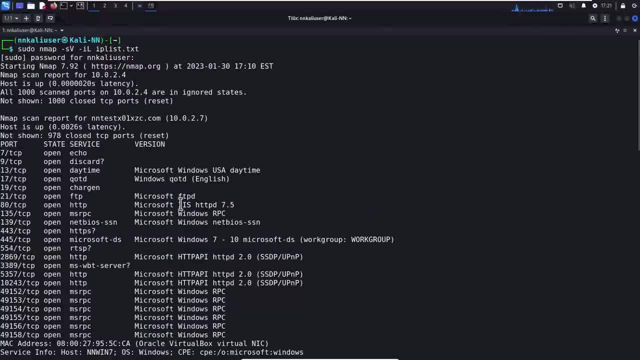 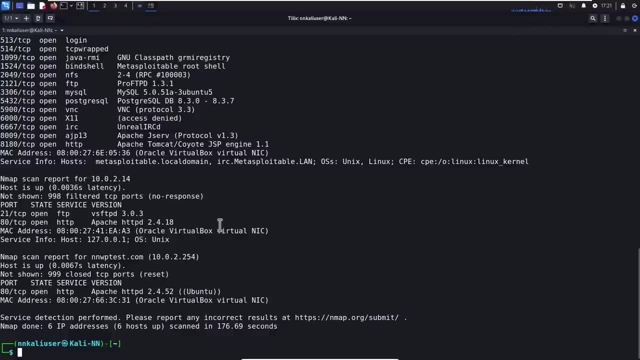 ton of them as well. uh, including is ftp, you name it. it also looks like it's running um smb, so the only one that looks good is the cali linux machine i'm on now, so that is how you could look for services and versions running, and that's going to be our kind of our bread and butter, for. 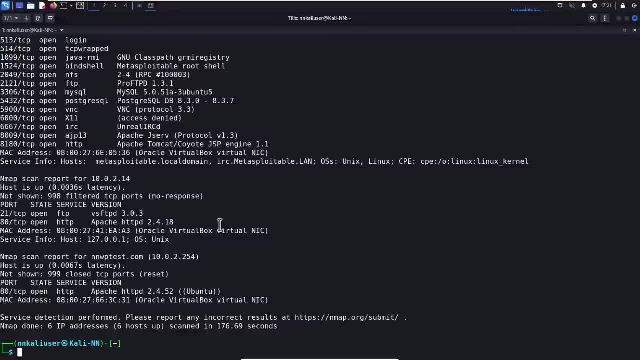 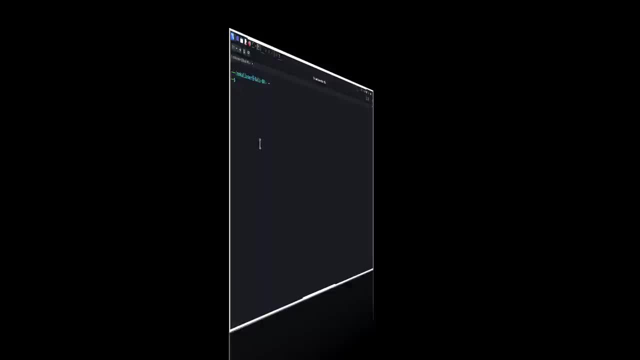 what we're looking for. but now, let's say we wanted to know, just to verify. you know it says Ubuntu here, but how can we take that a level further? and for that we're going to use this next scan, all right. so, following up with that service and version number, we want to know the operating. 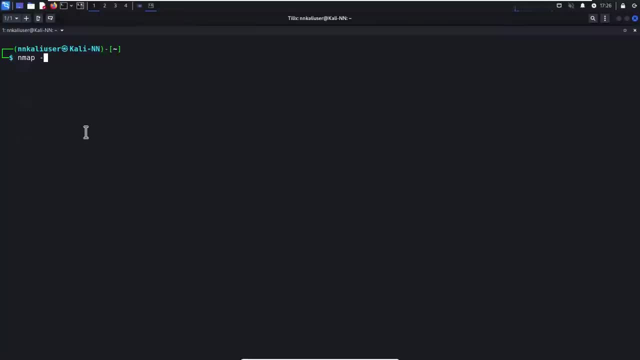 system and to do that, we are going to do an nmap dash. oh pretty basic, right, and then you would just do: you know, you know by now what we're doing. we're not doing that, we're doing this, we're just making sure you're paying attention. go ahead and hit enter. actually, we need to sudo this. I caught. 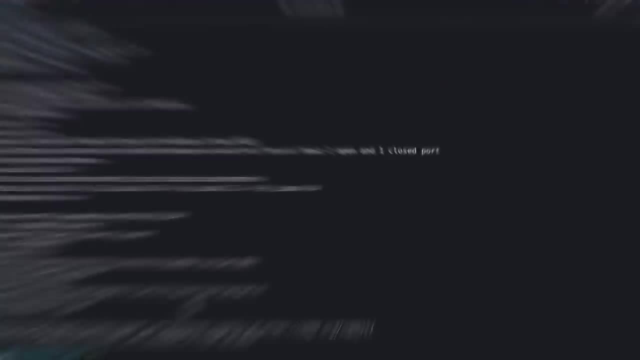 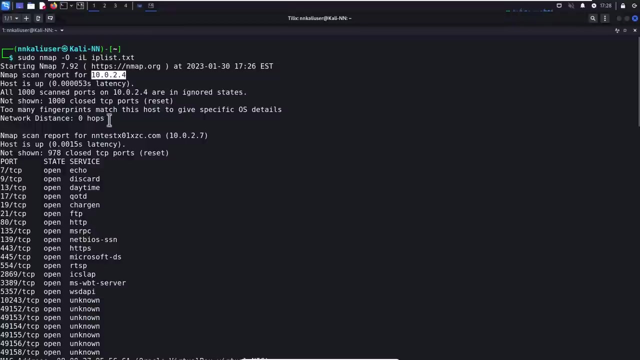 myself that time and hit enter and go ahead and wait for the results, and those results are in. so let's mix it up and go from the top down. this time started with my Kali Linux box and, no surprise here, it did not give it much information. that's what I would hope for. continuing down here we have 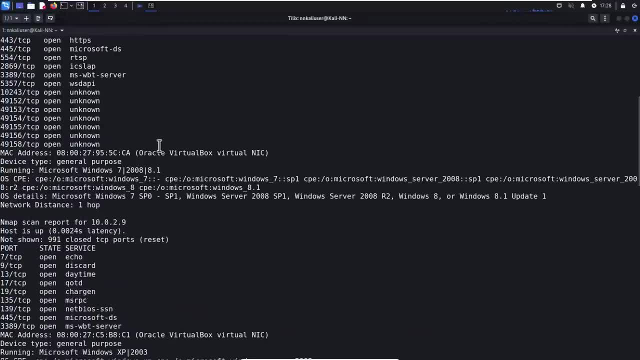 2.7, which, if we continue all the way down to the bottom, we can see that it identified it as a version of Ubuntu, and that's what I would hope for. continuing down here, we have 2.7, which, if we continue all the way down to the bottom, we can see that it identified it as a 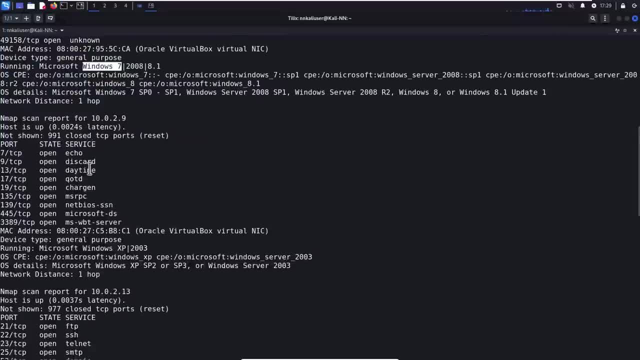 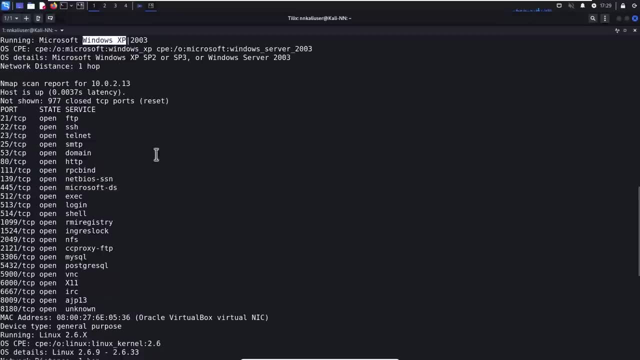 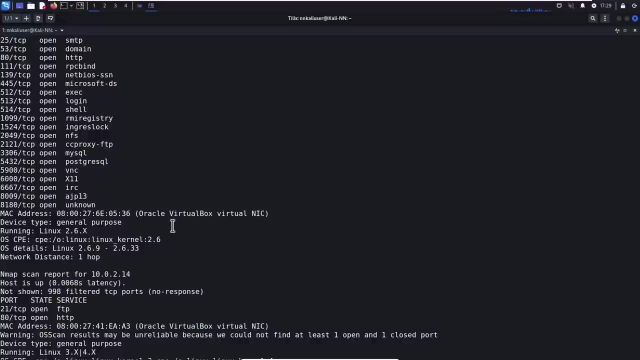 Windows 7 machine, and that is correct. it is running Windows 7, continuing down. 2.9 is running Windows XP, and that is also correct, continuing down. we have 2.13 that is running Linux. it doesn't tell us the exact release or distribution of Linux. 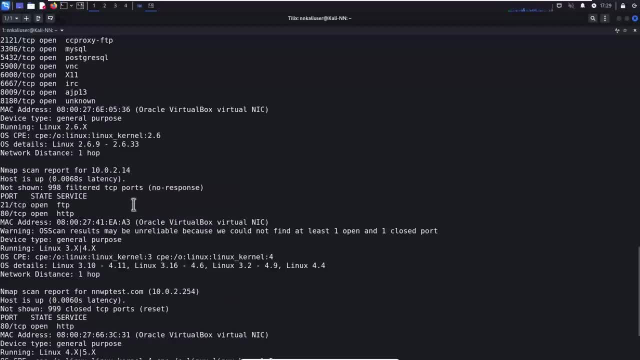 but it gives us close enough. we know it's Linux. 2.14 is also Linux, it's saying unreliable, and there are options we can do or switches we could put on to the command. I just ran to get these results that we can look into later, but for now we don't need that, we don't care so much, we just 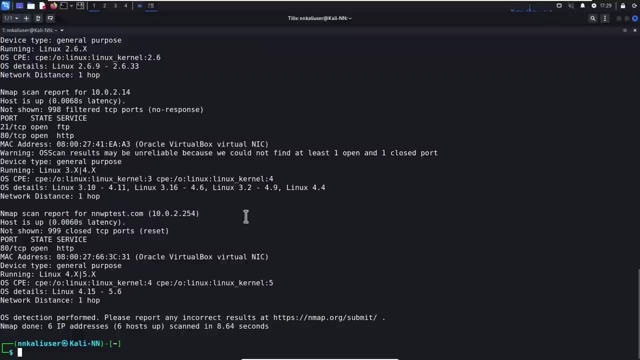 want to know that it's Linux and continuing done down, our last box is also Linux. so that's three Linux boxes and two Windows machines. so pretty good there. well, four because Kali Linux, but three that were open and returned results. so that's good. now let's move on to another. 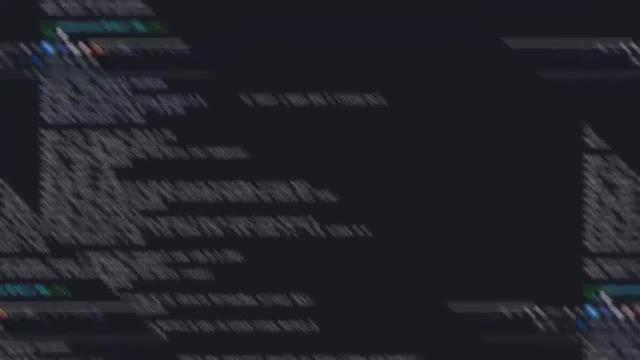 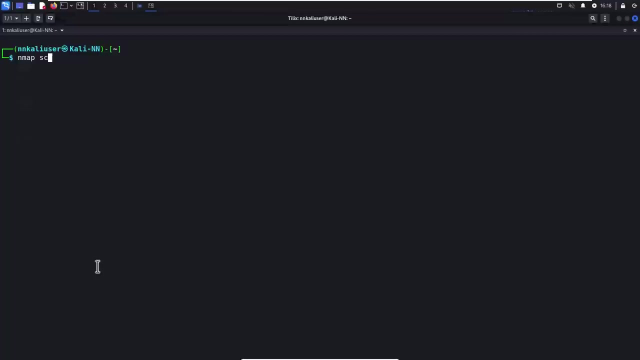 little technique we can do to either speed up or slow down our scanning, and that technique is pretty easy. I'm going to do it using the most basic of nmap scans, which is nmap, and I'm going to do scanmenmaporg, so we'll run it again, nmaporg, and here's where we're going to put in the switch. 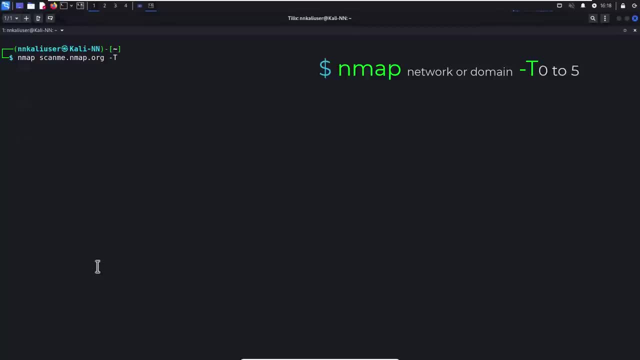 that's going to control the speed. it's going to be a dash t, and the dash t has a range from zero to five. zero being slow, what they call paranoid. five being the fastest, what they call insane. three is the default. three is the same as running the scan like this. so, for to test this, let's go ahead. 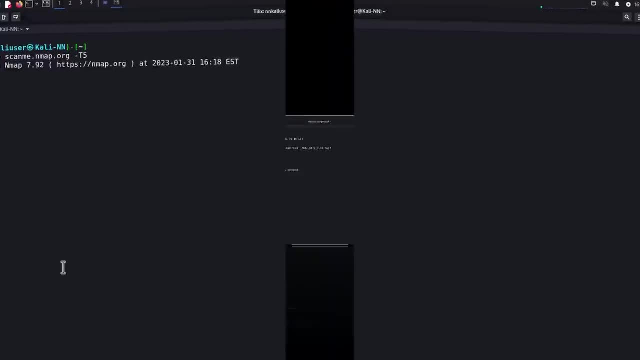 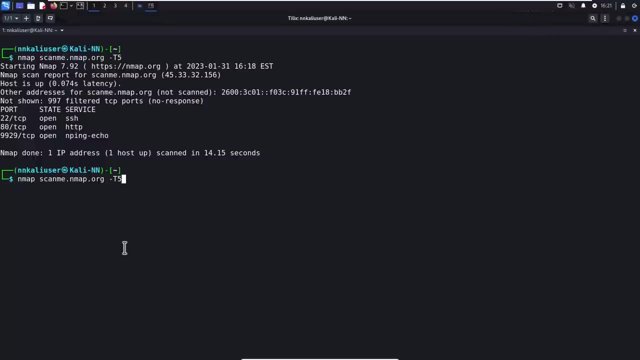 and put a t here and let's run it at a five and we'll see what it says. all right, and the scan finished and it took 14.15 seconds. so let's go ahead and do that same scan. let's try running it at a t3 and we'll let it run. all right, and here we go. so this one took almost double the interesting. 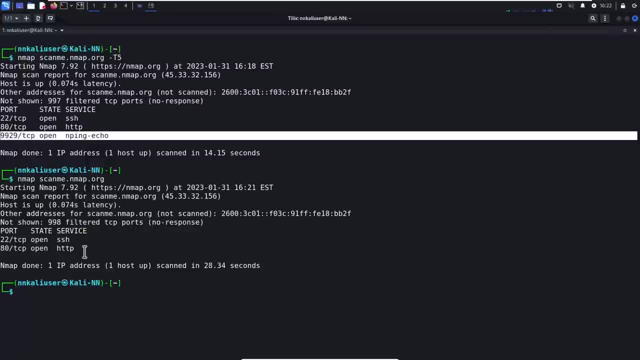 thing is this: actually picked up an extra port that this one didn't, and it's supposed to not work because it's not going to work. it will be a little bit more difficult, and let's do it the other way: the faster you go, the less accurate your scans are supposed to be. that's what that was going to be my 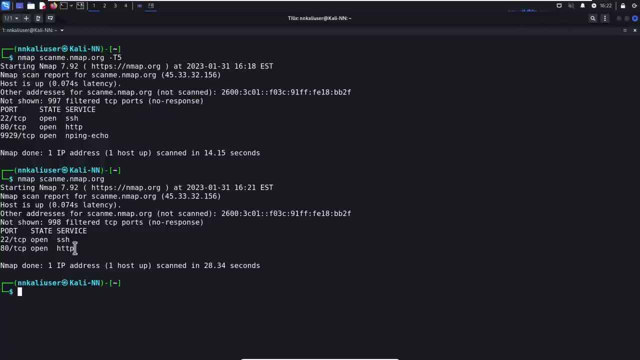 next point of why you would even want to do this, and that goes into: the quicker it's going, the less accurate it's going to be. the slower it goes, the more likely you're going to be able to go under the radar, you know, under the intrusion detection systems and things like that. but be warned when. 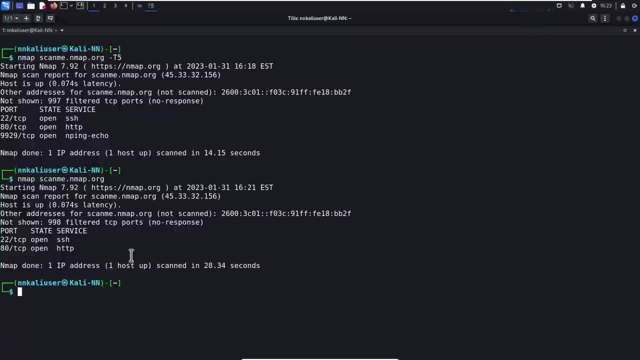 I say slower, I mean considerably slower. I once tried to do this and I used zero and it was at like and I hadn't had a single result and I just canceled it because it was too long. So just FYI, this is a way to do it, but I would, if you're going to do it, it should be for single hosts. 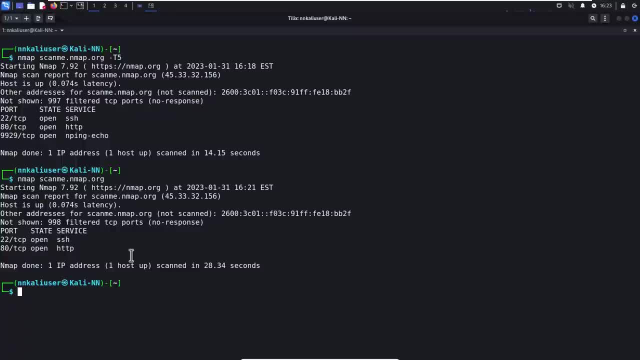 Do not run this against an entire network, or you're going to be there all day long using a zero. Now using a five, it wouldn't take as long, but you're going to set off every alert in the system, So FYI. So, with that said, let's go ahead and move on, All right, And continuing with the 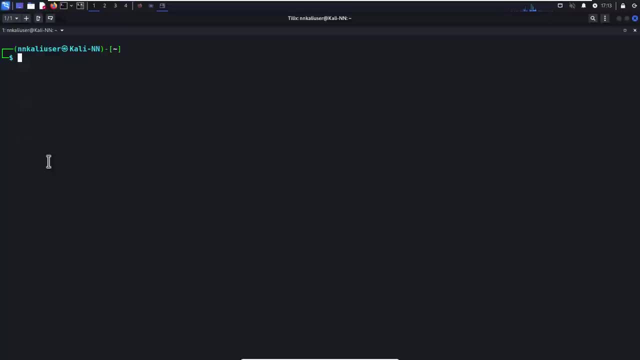 theme of trying to stay under the radar. you know we want to avoid detection. We're going to run what's known as a decoy scan and this is pretty cool. So what we're going to do is: first you need to be root, So we're going to go sudo or you could, you know, su to root whatever floats your. 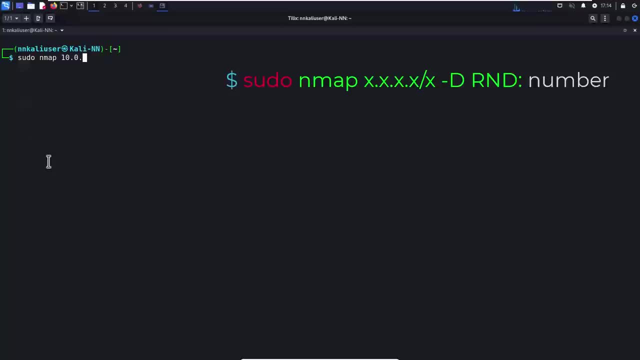 boat And then you're going to put in the IP or the subnet of the devices you want to scan- I'm just going to go against Windows 7 here, because we haven't picked on Windows 7 enough yet- And then what you would do is you would do a dash D and then you would do R and D, colon and the number. 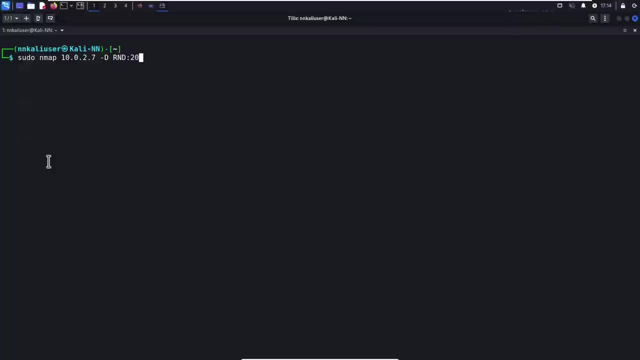 of decoy IPs you want to do, I'll go with 20,. you know let's go crazy. So we're going to go ahead and run this. But before we do that, let's go ahead and run this. So we're going to go ahead. 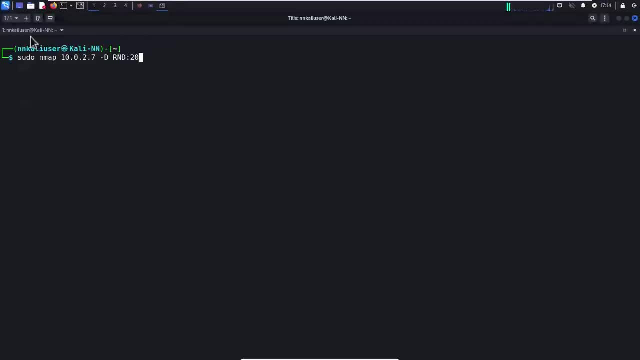 and do that. Why don't we do this? Why don't we open Wireshark And you can see what's going on as it's going on? So let's put these two side by side. If we can pull this off, we should be able. 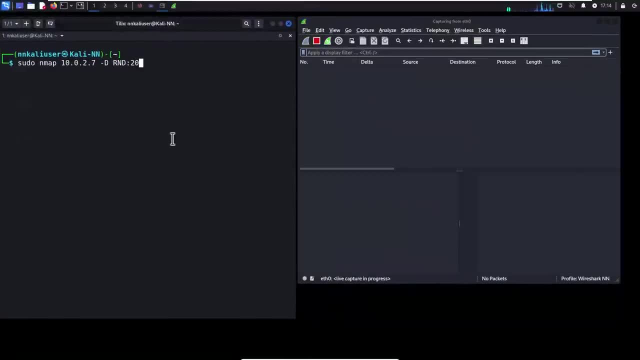 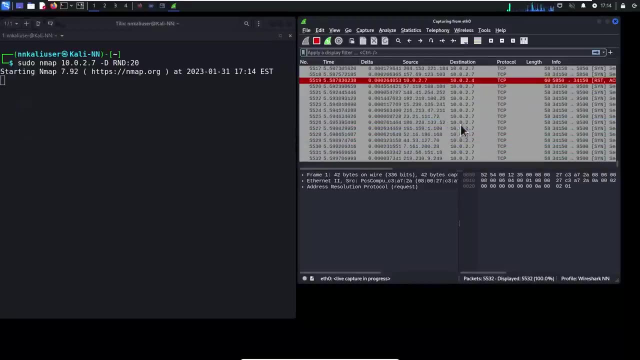 to. All right, let's go ahead and open ETH0.. And let's go ahead and run it and see what we get. And boom, as you can see, the outgoing 2.7 is getting flooded by all these source IPs. So now, 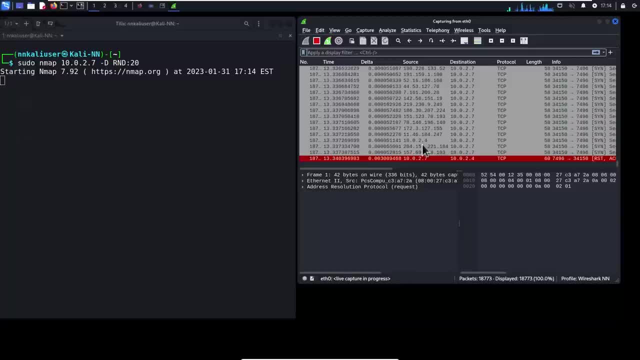 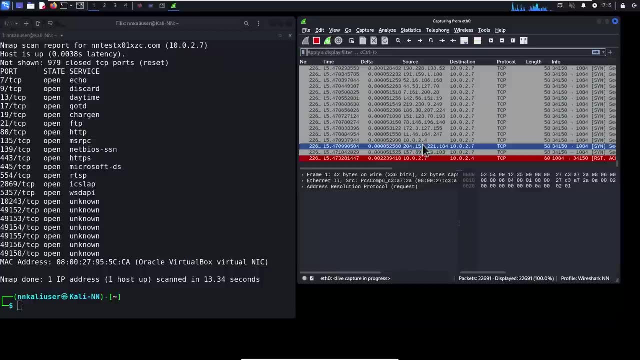 while we're not completely off the log, we are now in the log with 20 other IP addresses, Which will make it a lot harder to pick out one specific IP address. Pretty cool stuff right Now over on our end. we got the results we wanted and we don't notice much difference. This is more. 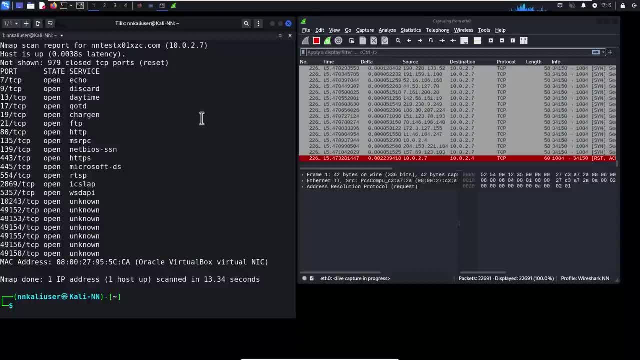 going to be for the destination side. You're not going to get any different results at all. But that's good, because we weren't trying to get different results, We just didn't want them to know where we were. So, mission accomplished, right, Right on. So let's go ahead and move. 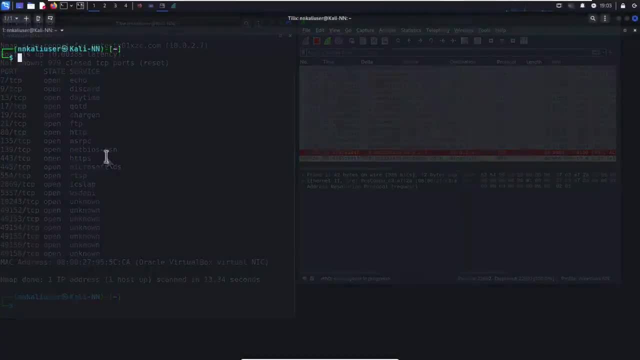 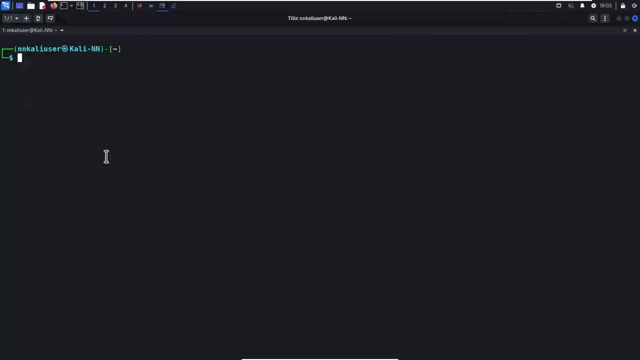 on to another way to try to avoid detection. All right, the next technique I'm going to show you is going to be to optimize the order that your scan is performed. By default, if you were to pick a subnet, it's going to start sequentially and work its way through, And that can be pretty easy. 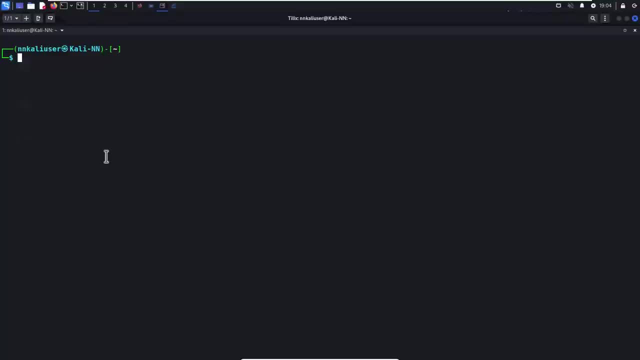 for you know, intrusion detection systems and other defensive controls. to pick up, because you're going from one host to another. This is going to go from A to D to C to F and all over, instead of going A, B, C, D, E. So how to do that? Pretty simple, We're going to go end map and we're just. 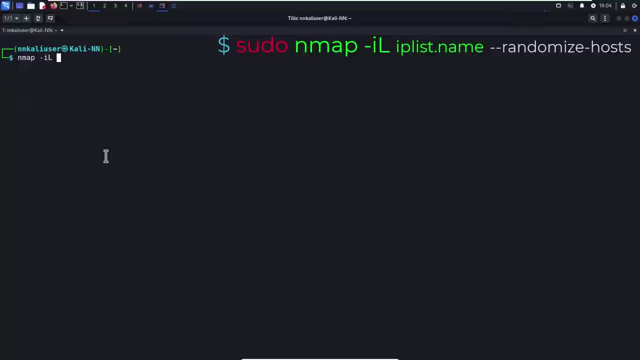 going to go IL And we will go ahead and pick a subnet And we're going to pick a subnet And we will go ahead and pick a subnet And we will go ahead and pick a subnet And we will go ahead and put an IP list dot text And at the end all you need to do is add randomized hosts, And I believe 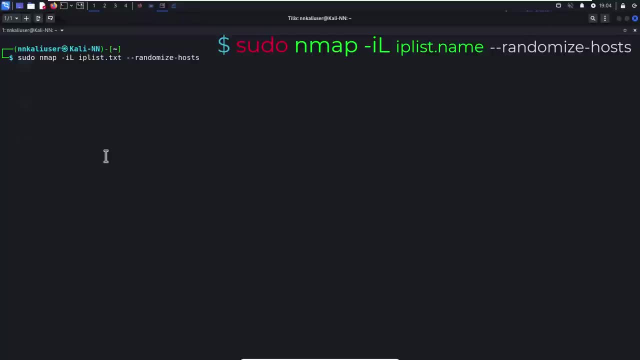 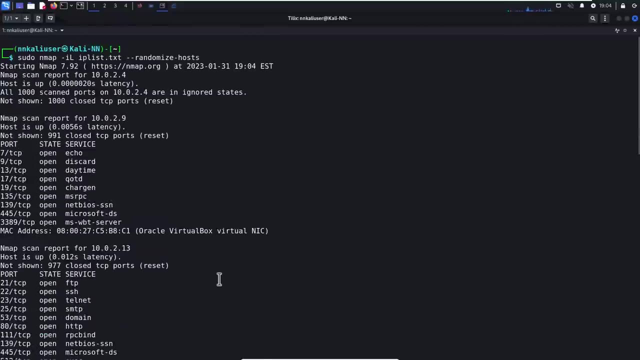 we need to be root for this, So we're going to throw a pseudo in there And we'll go ahead and hit enter, And now we'll wait and see what happens. All right, and the scan completed, Let's go up and take a look. This should go from two to seven to nine And, as you can see, it went from. 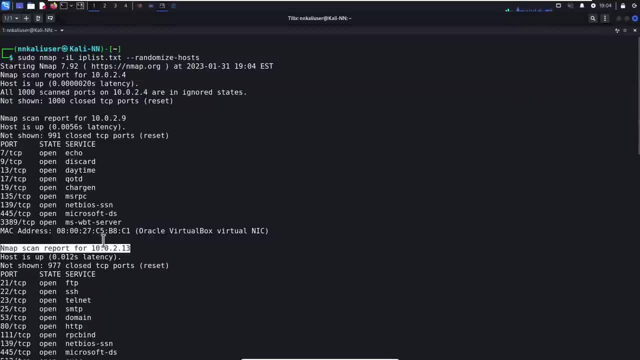 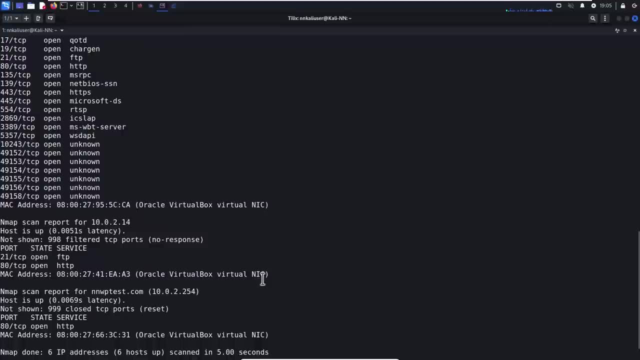 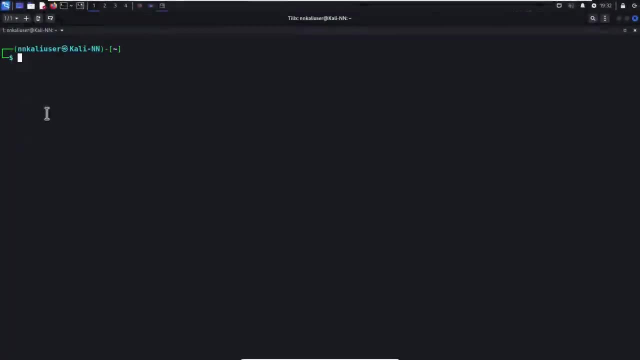 two, or from four, excuse me- to nine, to 13,, to seven and down to 14, and ended up with 254.. So, as you can see, it did exactly what we asked it to. So that's another technique to keep you off the radar. All right, and the second to last technique. 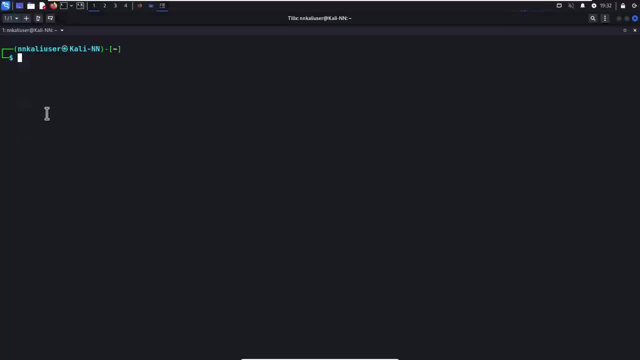 I want to show you to try to avoid detection is going to be how to spoof your MAC address, And this is pretty straightforward. We're just going to go pseudo end map and enter the IP address of the device you want to scan. We'll go ahead and run this against our Kali Linux box here, just to. 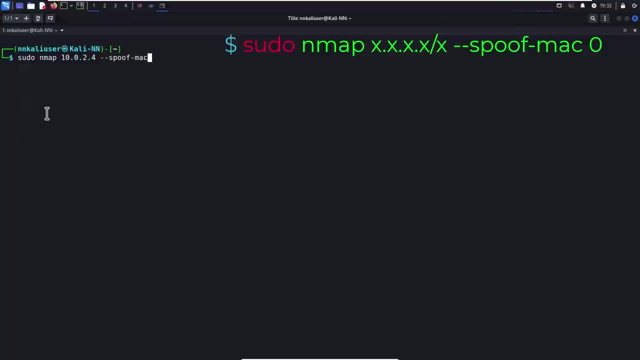 see what we get. And then what we're going to do is we're going to go spoof MAC And we're going to enter a zero to randomize the number. If you wanted to actually fill it in, you could go ahead and do that as well, But I don't really see what the point of that would be, So I'm going to go. 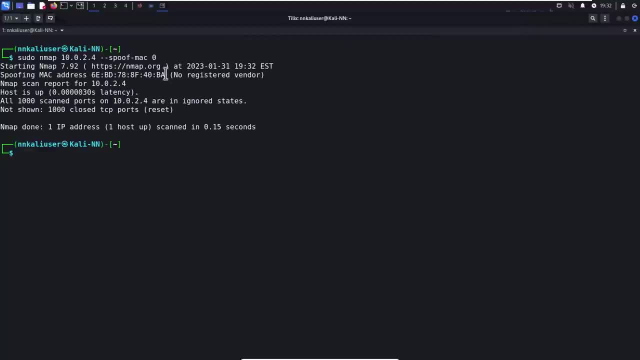 ahead and run this and see what we get And, as you can see, here's what it went with. That's the MAC it picked for us, scanned and we knew this box had no open ports because it's pretty well-hearted. So what we want to do now is check to verify that it didn't really use our real MAC. And here's our 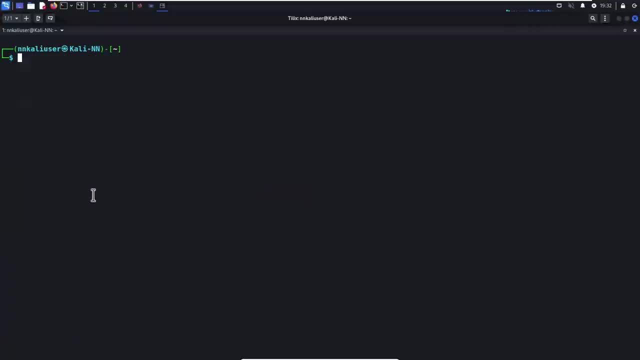 real MAC. So no, it did not. So pretty straightforward technique. Nevertheless, it can help keep you off some detections, if they were, you know, actually blocking MAC addresses instead of IP addresses, Because unfortunately there's no easy way to spoof your IP address short of using 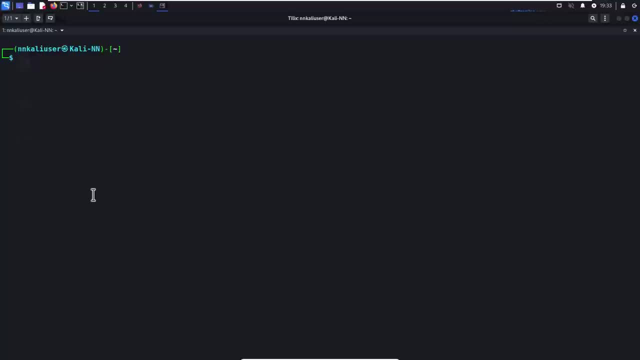 something called IP change, which uses a proxy, And it's out of the scope of this video. Maybe I'll do another video at some time on that, But that's a little more technical. But nevertheless, this is one more technique Moving on to the last technique for avoiding detection. 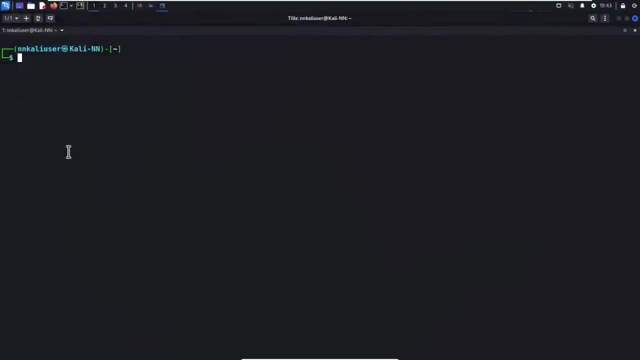 For the last technique I want to show you on trying to avoid detection. we're going to do something. next. We're going to do something that's going to help you avoid detection. It's going to be known as packet fragmentation, And what is that? That is going to be where we're 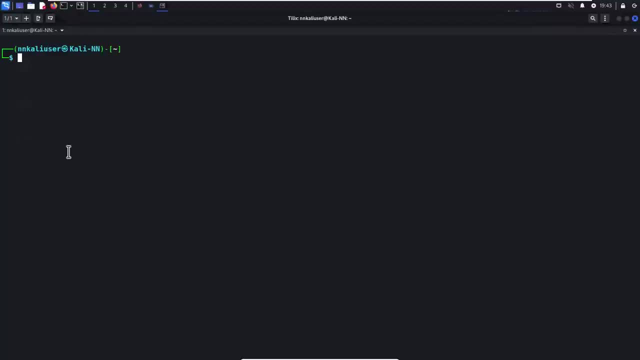 going to take our packets and fragment them into smaller packets, And the reason we do this is we're hoping the smaller packets will be able to avoid detection. They'll be able to, you know, bypass those content filters, firewalls, intrusion detection systems and things of that nature. 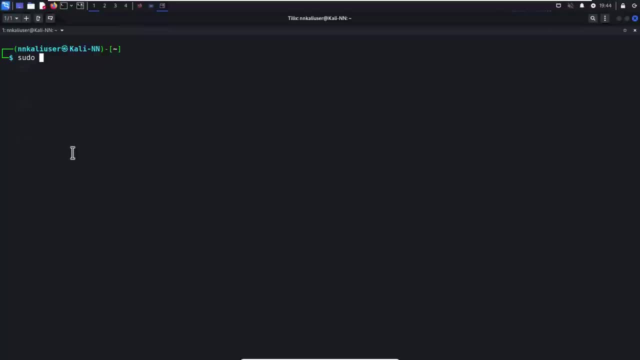 So let's go ahead and do it. And to do it, it's very basic. We're going to go nmap or sudo, nmap, always sudo, And then we're going to put in the IP address. We'll go against nine. 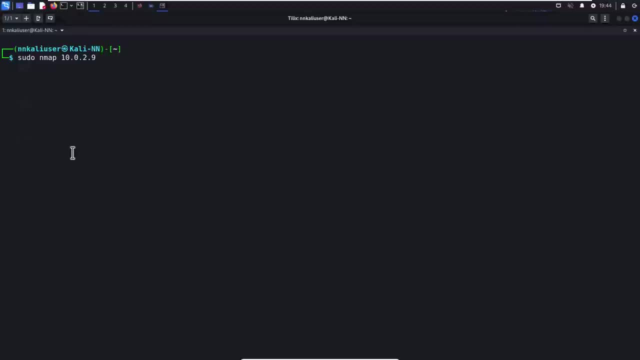 because we've picked almost every other server we have here, And then what we're going to do is we're just going to put a dash up at the end, That's it. But before we do it, let's go ahead and open up Wireshark so we can take a look at what it looks like going out. So we'll do that. 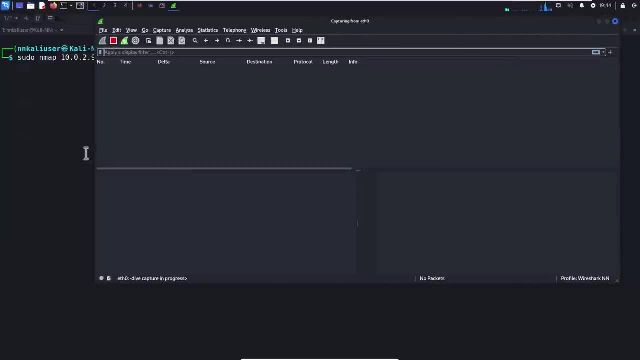 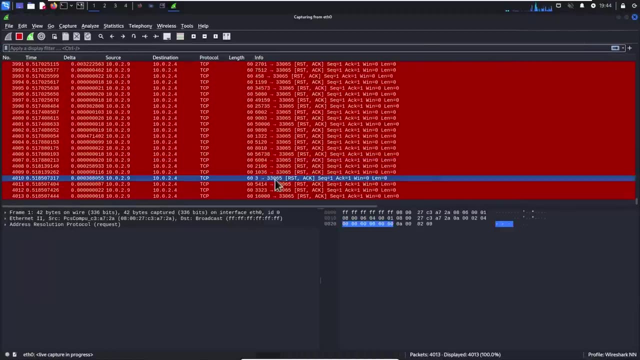 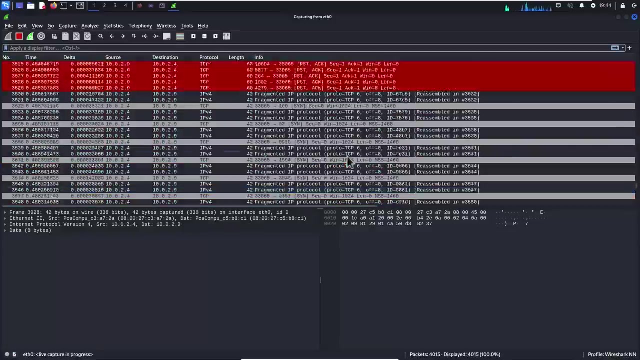 Go ahead and do that And let's go ahead and hit enter Done. Go over here And this looks normal, right, But check it out, Oops. scroll by so fast. See this. This is a fragment that was broken up And all these all the way up here And you can see it goes all the way up there. 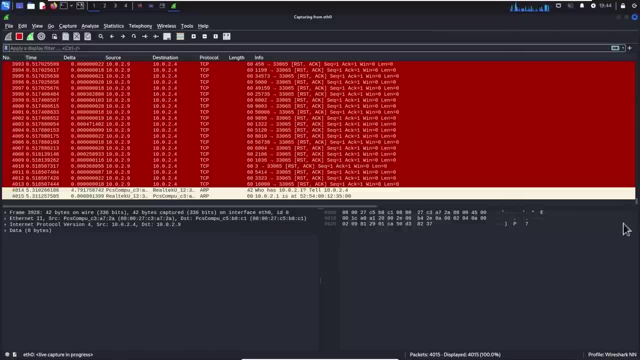 So in my personal experience, I would say this helps maybe one out of every five times. This isn't like the oh, this is going to work every time. It's going to get by the detection systems. It's not all that great, But you know what? It is another tool And it's definitely 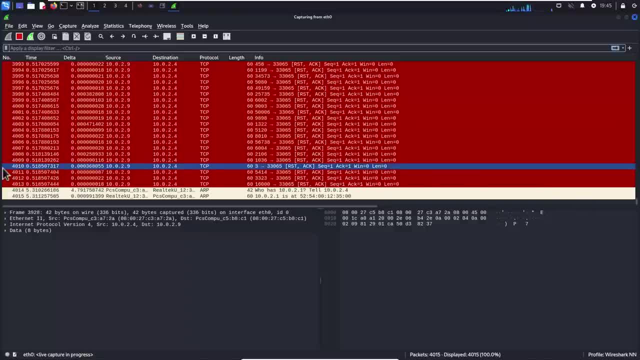 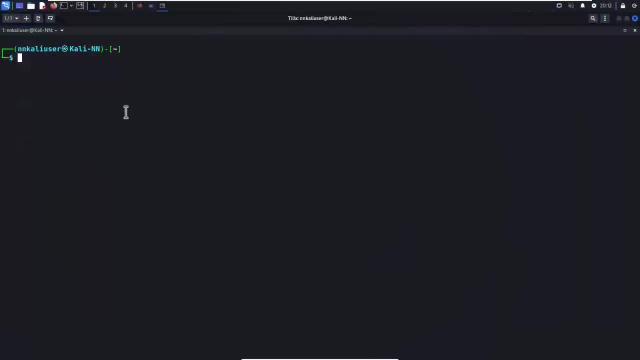 worth keeping in your arsenal. So, that said, let's move on to testing these services for vulnerabilities. All right, At this point, if this were a penetration, let's see what we've done. We've discovered the devices on the network. We have singled out the. 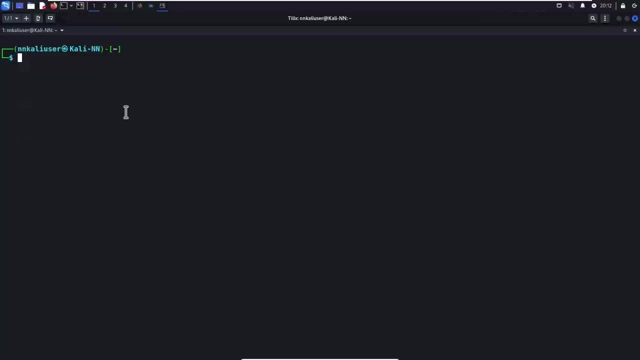 devices we want. We have singled out what ports were open on them, what services were running on those ports, what versions of services were running and what operating system. So we have compiled all this data. Now, at this point, we're ready to go to the next level, And what we're 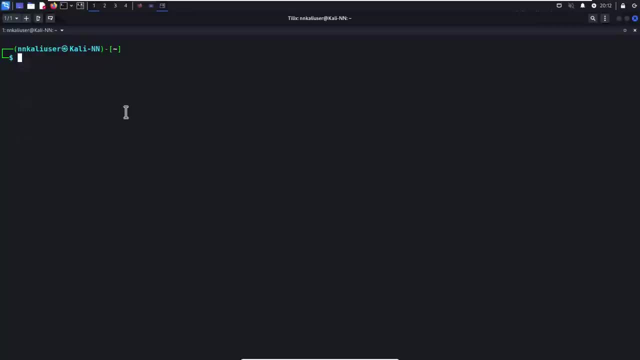 going to do at that stage is we're going to now test to see if there's any known vulnerabilities to those specific service versions running on each of those hosts, And to do that we're going to go ahead and do a little bit of storage and map scripting And to get scripts you can either. 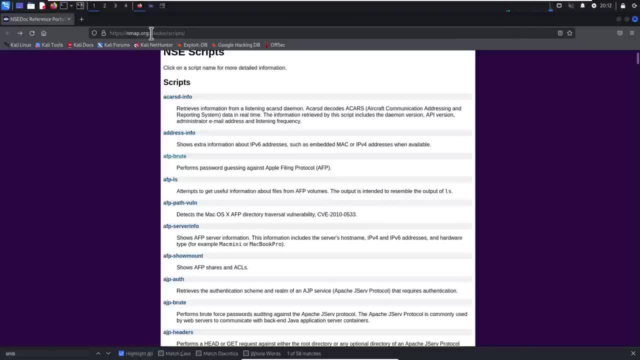 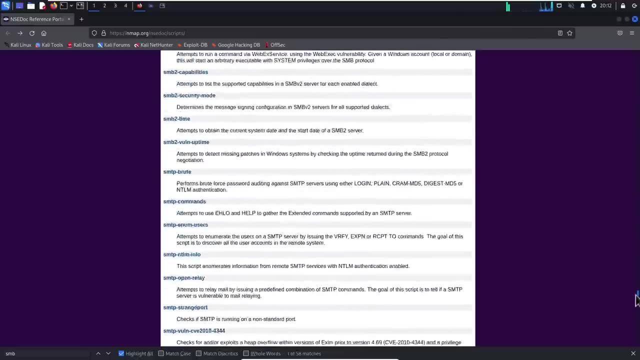 go out to their website Right here, I'll show you. You're just going to go to mmaporg. I'll put the whole URL in the description And here you're going to get a listing of scripts, a really long listing of scripts of all different kinds of built-in scripts that you can either download by: 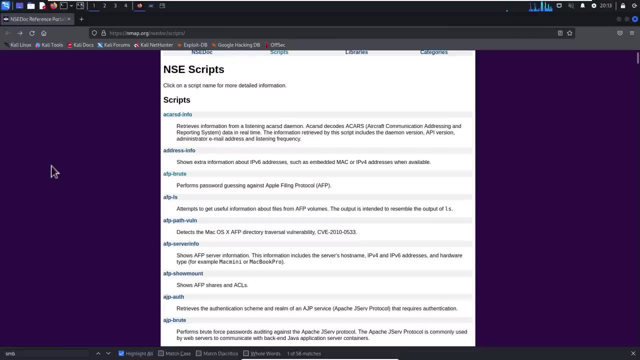 clicking on them and hitting download. Some of these are actually already pre-built in And some of these actually come with different distributions of Linux, But if, for whatever reason, it's not, you can go here and download them, So that will work for everyone. Windows, Linux, you name it. 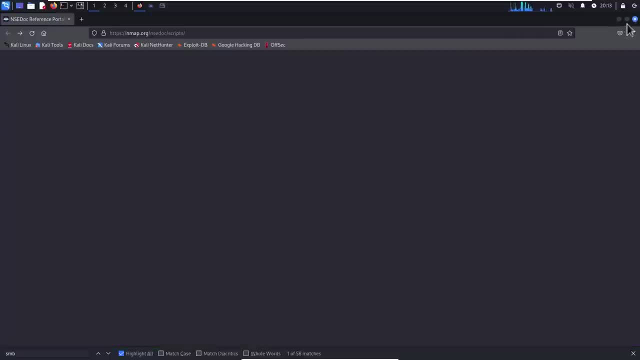 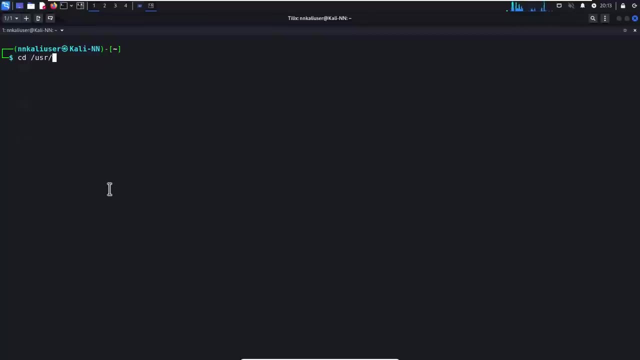 You can go here and get them. For those of you on Kali Linux, you're in luck, because they actually come pre-installed, or pre-loaded, I should say, And to get there you would just go to this location And actually one more folder in here. So if we do this, you can see well. 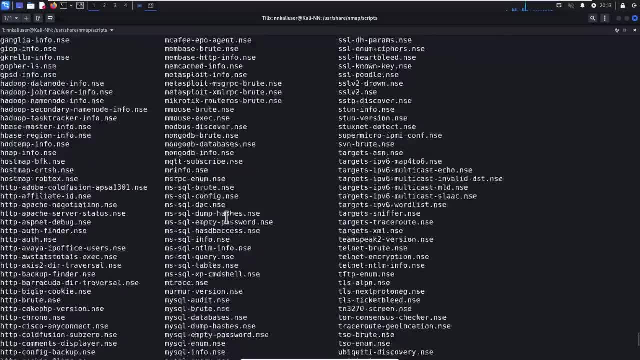 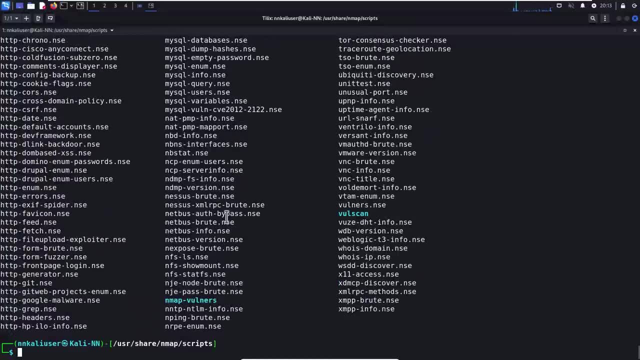 actually. maybe this will give you a little bit better view, But you can see they're all there for the most part. Again, if one wasn't here, you could go up and get it from the website. So that's where we're going to get the scripts. Now let's move forward and show you some of the 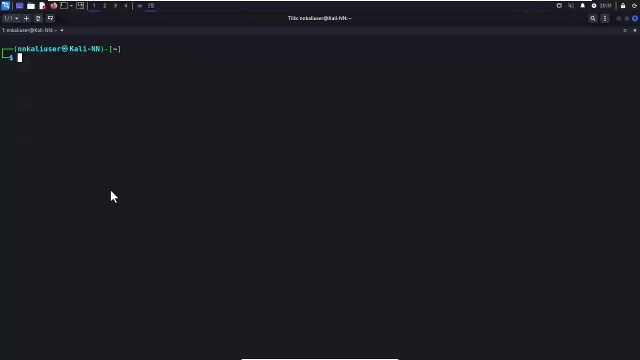 most popular ones to look for vulnerabilities. All right, And before we get to our first script, I'm just going to ask, out of the kindness of your heart, if you could smash that like button. if you are enjoying this video or learning anything, I would greatly appreciate it. 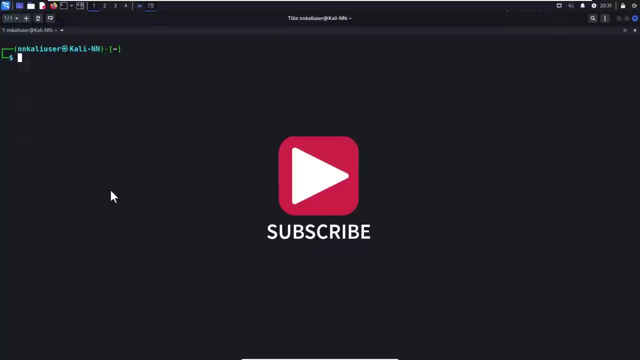 If you want to one-up me on that, go ahead and subscribe for future content. We're trying to get a lot of content out there And, believe it or not, about 80% of our viewers don't subscribe, So they never get the notifications again and maybe they never. 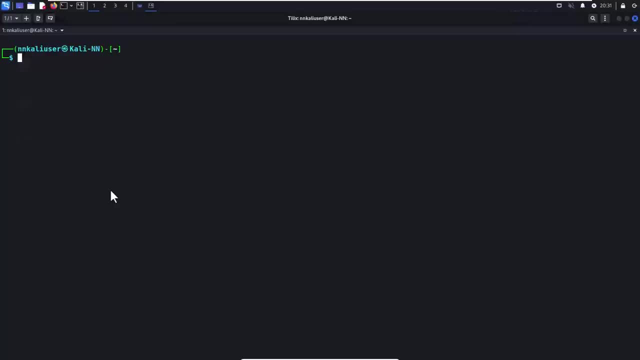 come back to see all the great content I believe I'm putting out there, So that, out of the way, the first script that we're going to run is one that's going to go out and look for SMB vulnerabilities on our two Windows machines which we have, an XP and a Windows 7.. So enough. 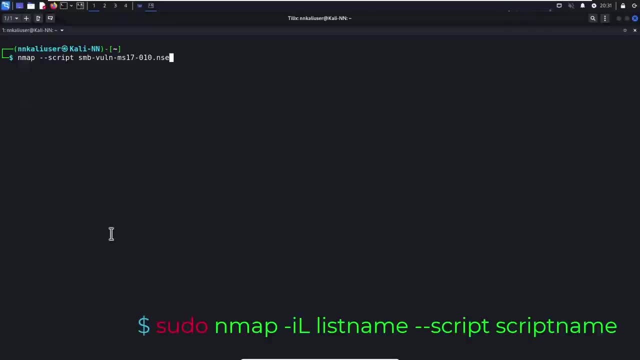 chit chat, Let's get to it. We're going to go ahead and run this command out here. We're going to need to change it up a little bit to add what we want to scan. So I am, of course, going to put. 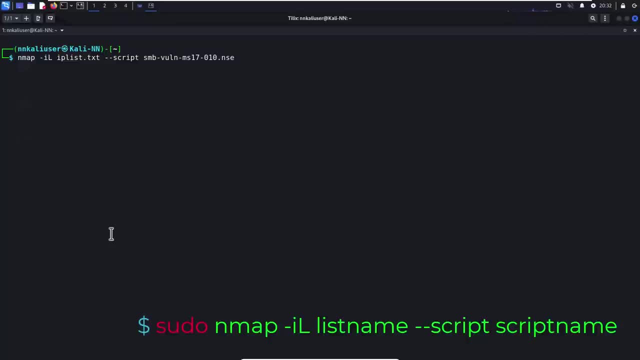 this little overkill. This is going to scan all devices, but you know what? I don't care if it runs against the Linux machines. We'll at least get the Windows devices while it's scanning that. So that's cool. You would probably want to be specific in each device, but for this video. 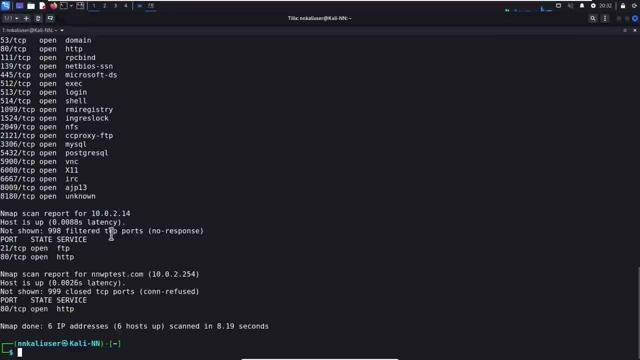 I'm just going to run this list because, be honest, it's been a long video, So we're going to let it run and we're going to see what we get. So let's scroll up here, Let's go all the way up to the top. 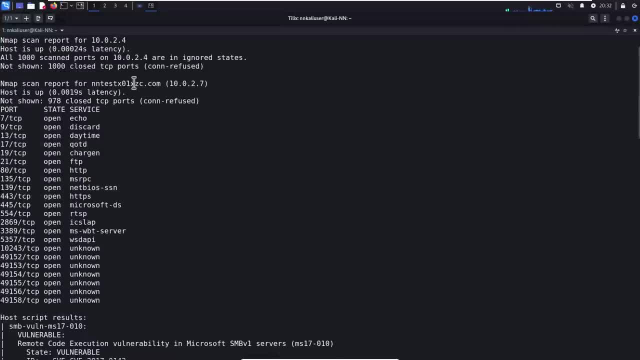 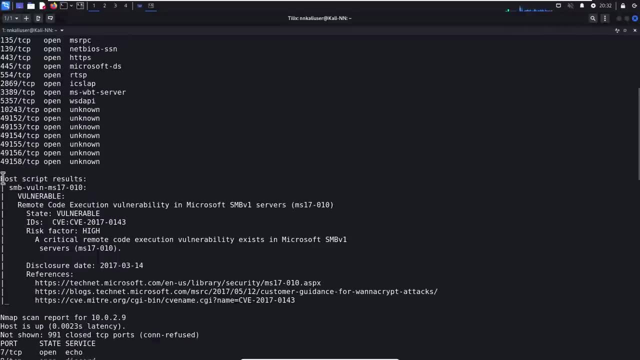 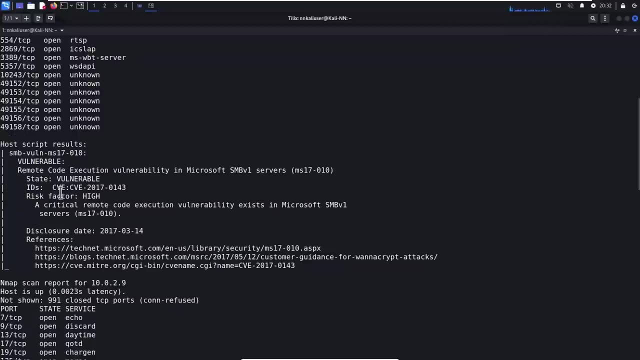 and we can see we got some hits there. So obviously, the Linux box: nothing. This is our Windows 7 machine Scrolling down here. Here we go, Right. here is the vulnerability we were looking for, and it's showing it is vulnerable. So that is one we would then, and maybe we'll do it at the end of the 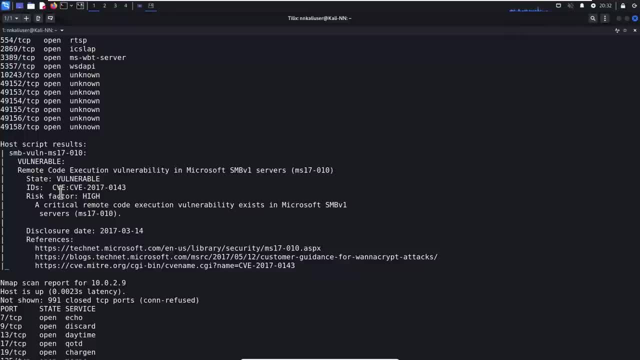 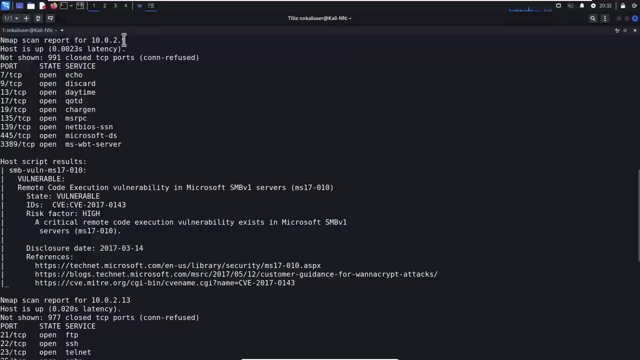 video. We would then, you know, go and take it a step further and maybe open Metasploit and see if we could actually exploit that vulnerability Scrolling down same thing on our Windows XP machine. So we found those two vulnerabilities. Let's go ahead and check a different vulnerability. 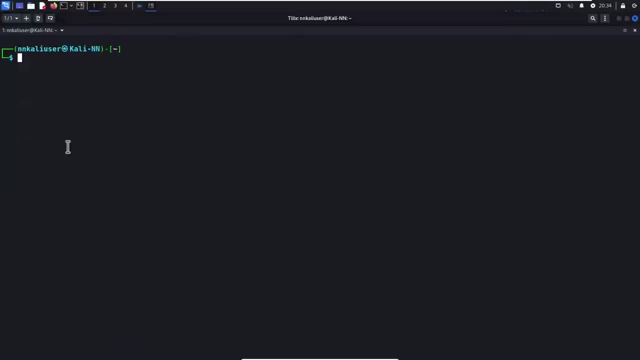 All right. Next, we're going to go ahead and scan for a known vulnerability with VSFTP, which we saw at the beginning. Remember how I said: I think there's a vulnerability out there. Let's go ahead and find out if there actually is. 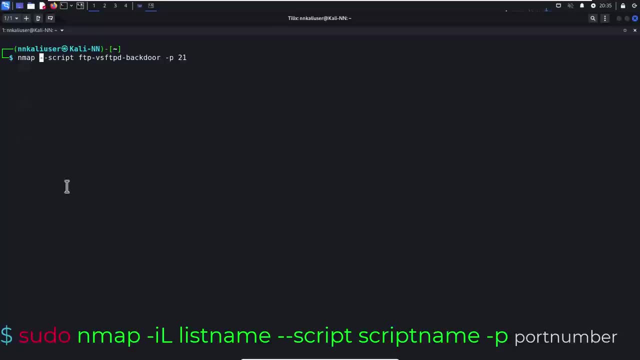 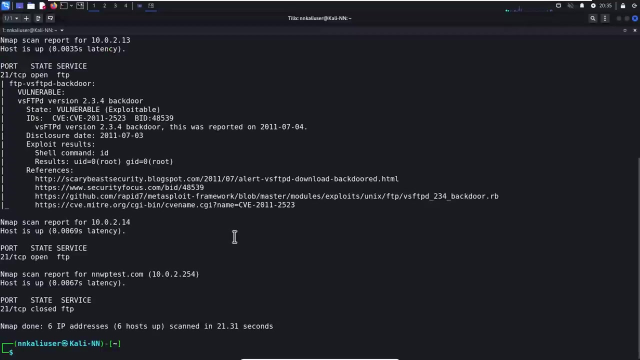 So again, we're going to go ahead and paste this in, We're going to change this and we're going to add our IP list and we're going to go ahead and run it. See what we get. All right, And here we are, it's done And we can see. right, here we have one, And, of course, 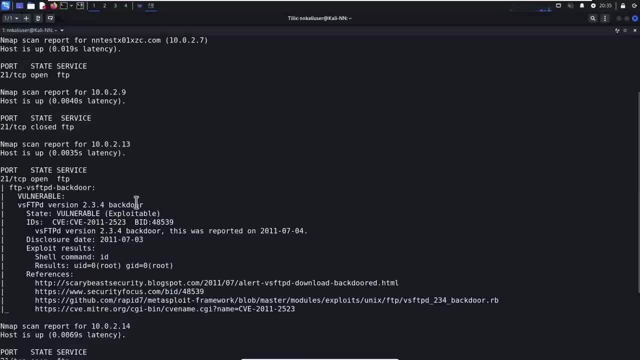 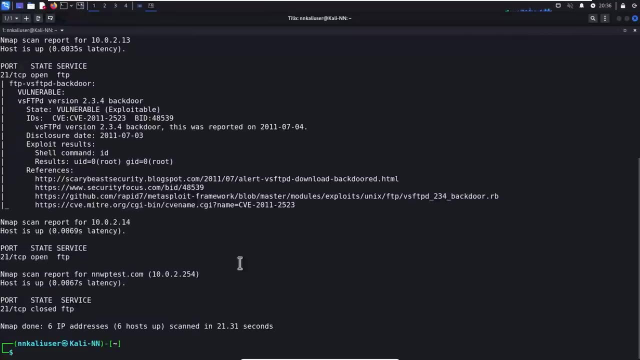 lucky number 13,. surprise, surprise. I thought we'd actually get two hits, because I remember we saw this twice, but apparently that other version is not vulnerable, but this version is. So 13 is vulnerable to a backdoor here. So that's that. Let's do one more. And for the last script I want: 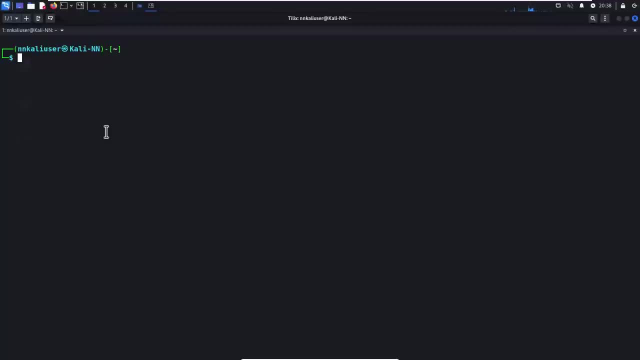 to show you. we're going to use a script known as vuln, And what vuln does is it actually scans for all the known vulnerabilities in that category. So instead of individually scanning for, you know, FTP or SMB or SSH known vulnerabilities, it's going to scan for all of them at once. So this: 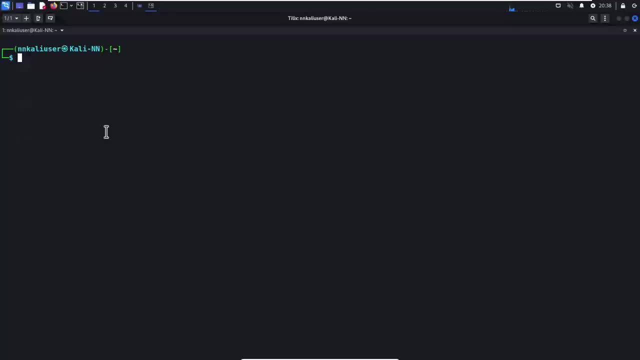 would probably be the easiest if you wanted to scan a broad range of vulnerabilities and not a specific one. And to do that it's really easy. We're going to go Nmap and we're going to do IL for our list, And then you're just going to do script and you're going to type in vuln, short for. 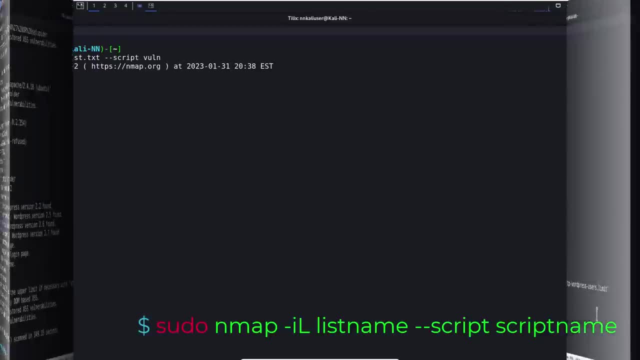 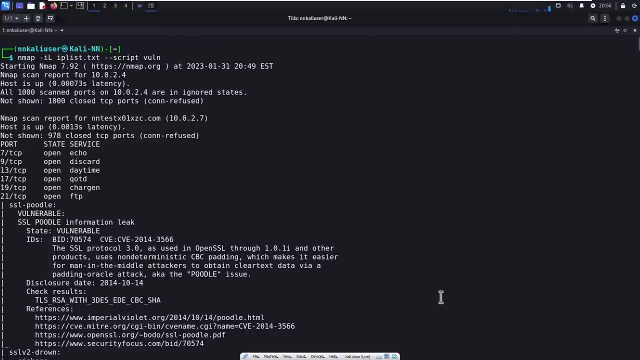 vulnerability. hit enter and give it a little while and we'll check the results. All right, And the results are in and it took a little under six minutes. So let's scroll up and look at all what we got And starting at the top, 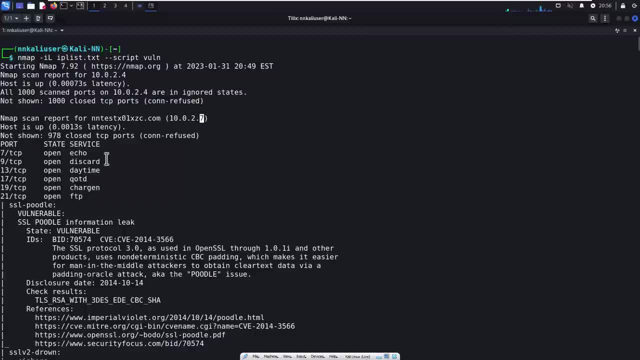 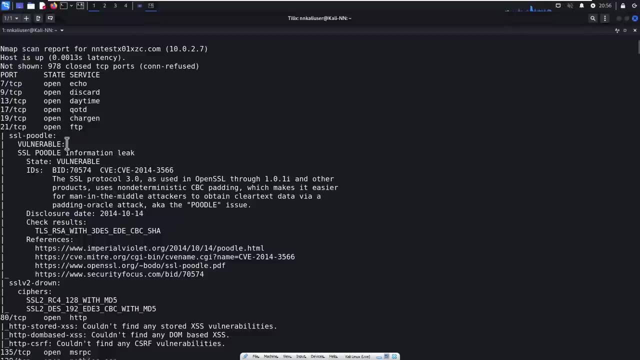 with our Windows 7 machine. scrolling down, you can see it started at the typical ports, worked down, and it looks like the first thing it discovered is a vulnerability with poodle. This is going to allow for a man in the middle attack, I believe, Yeah. So it found that scrolling down. 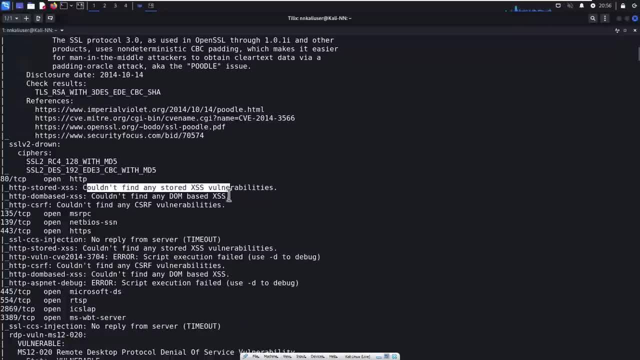 It does tell you that there was no cross-site scripting vulnerabilities found or cross-site request forgeries. So this doesn't have to just be used by pen testers. This can also be run by net admins- system administrators- to go out there and see what is on your network. 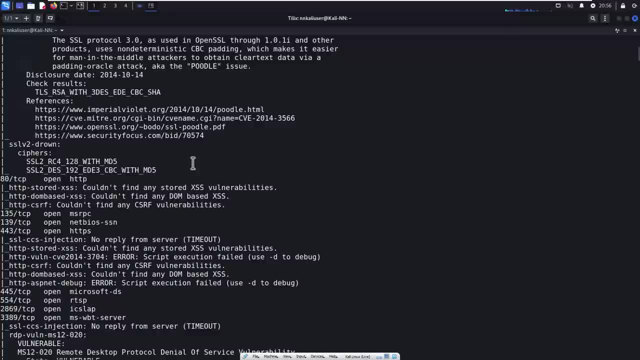 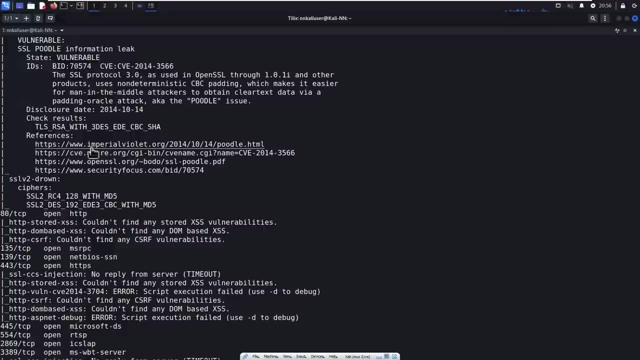 Why wait for a pen tester to come in and tell you You could do this on your own? And if you're doing it from that angle, you can also check out these websites that will give you remediation techniques to use if you wanted to go out and do it that way. So just remember this isn't just for pen testing. 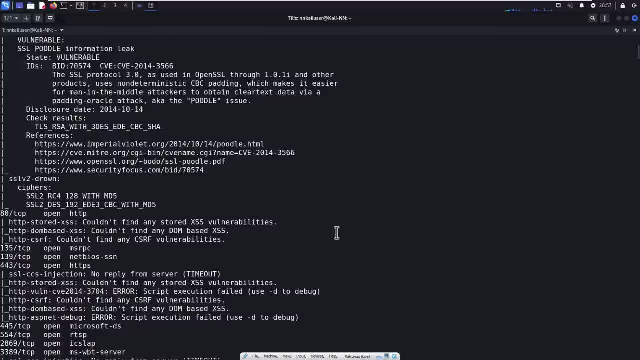 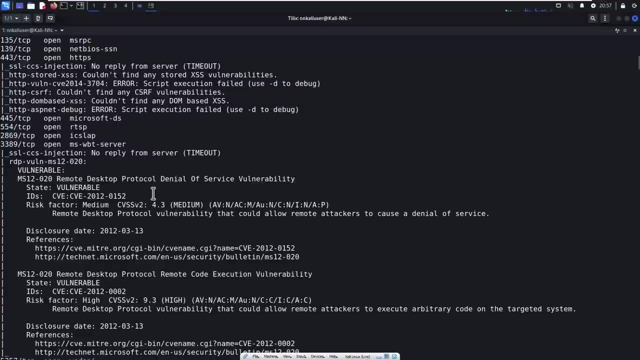 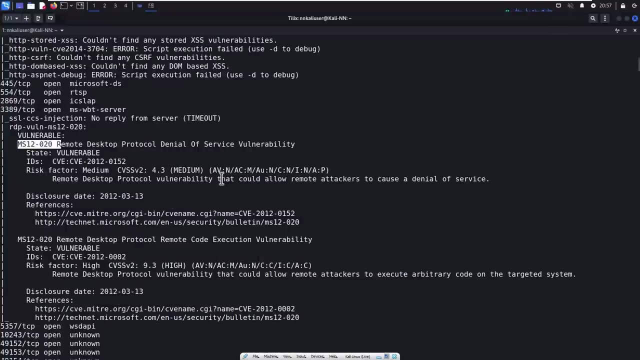 The focus of this video is on pen testing, but this can be used in multiple different ways, So continue on down. It looks like it's also vulnerable to this vulnerability right here. remote desktop protocol and continuing down, lots of vulnerabilities, So let's continue. 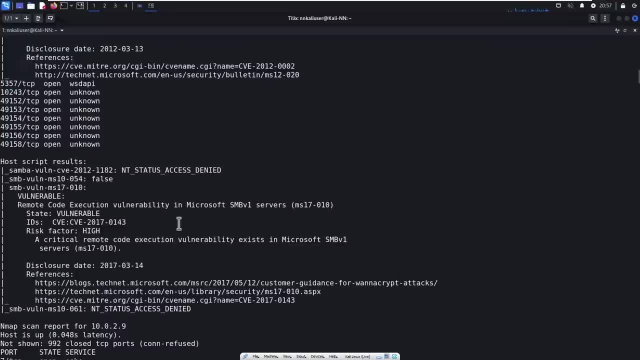 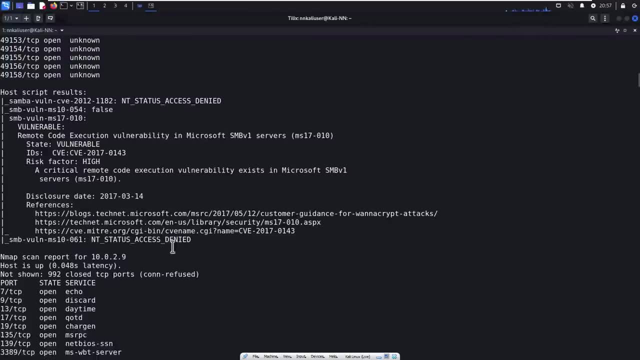 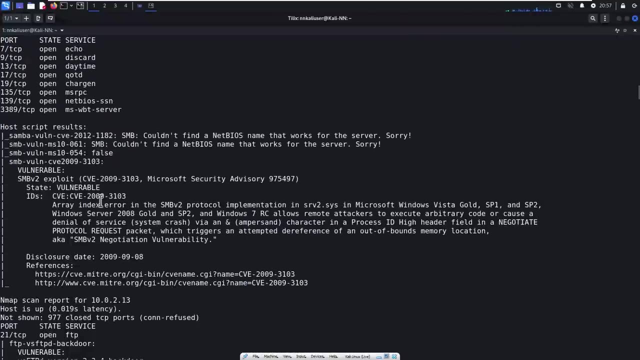 down here to our next machine here. This is going to be the SMB vulnerability And wow, Okay, So lots on that machine. That is not a pretty machine. And then we're going down here and I believe this is our Windows XP machine And this one was vulnerable again. 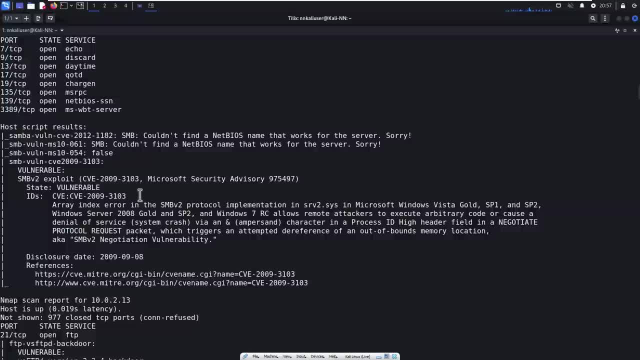 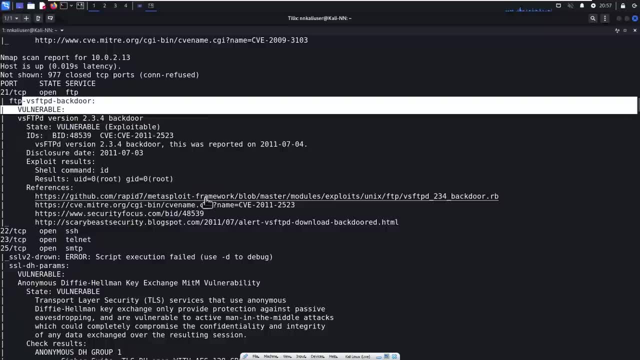 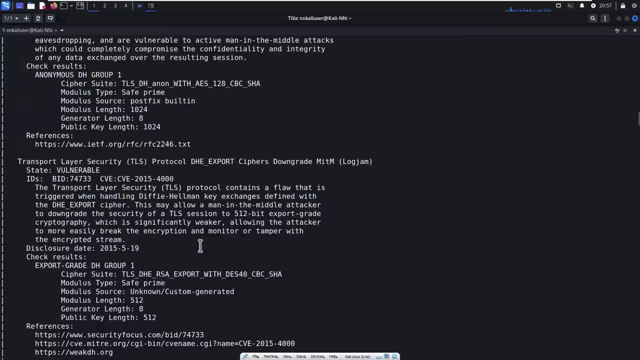 right here, another SMB vulnerability, And I'm just going to kind of continue on down here because we will be here all day. Again, this is that FTP vulnerability we saw. This is a new. another vulnerability with the SSL version. they're running and continue on down. 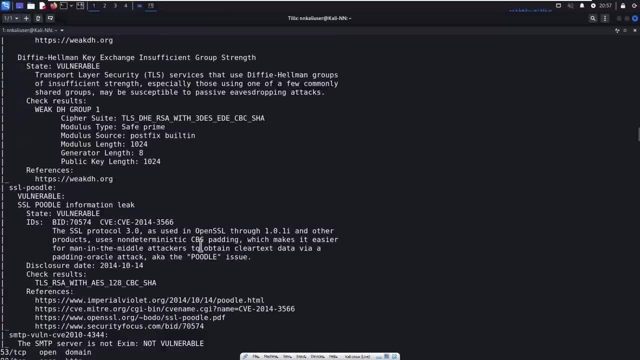 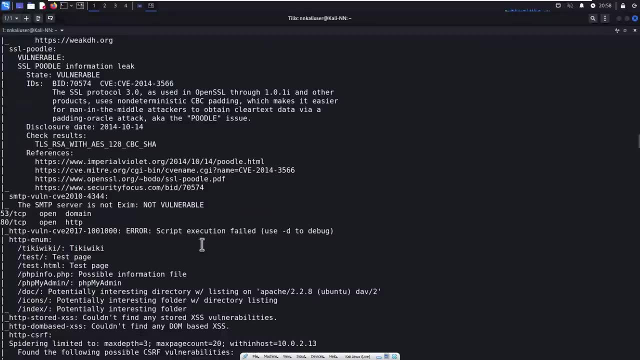 There's lots of vulnerabilities in these machines, And a lot of that is by design, obviously for this new machine. So that's why we're going to put machines out there that were going to give us some results, Otherwise, how would we know what to look for? So, as you can see, we can continue on all day. 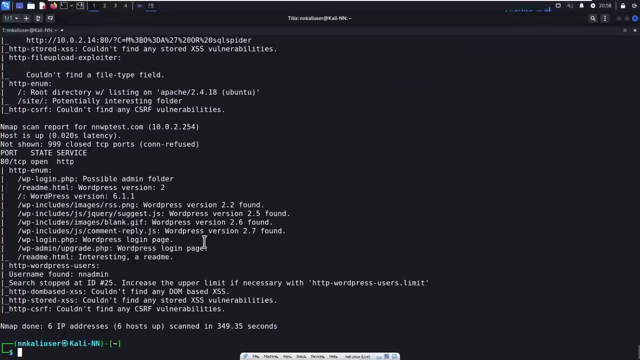 long. There's a lot of vulnerabilities to go through here. So that all said. I think that kind of wraps up the video from Nmap perspective. Now let's say we want to take this one step further. right, Let's say we wanted to actually see if now we could exploit one of the vulnerabilities. 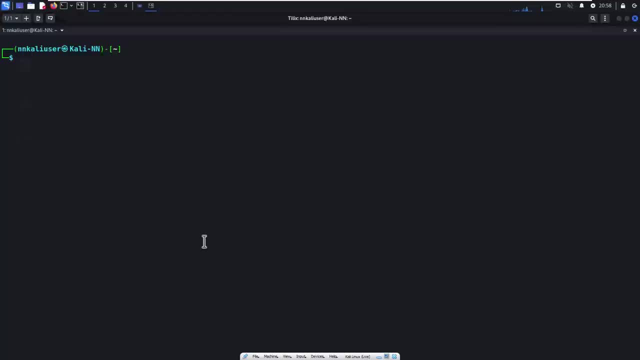 we discovered. So as a little bit of a bonus here, I'm going to show you how we could see if that's possible using Metasploit. So let's get to that, All right. And if you don't know what Metasploit? 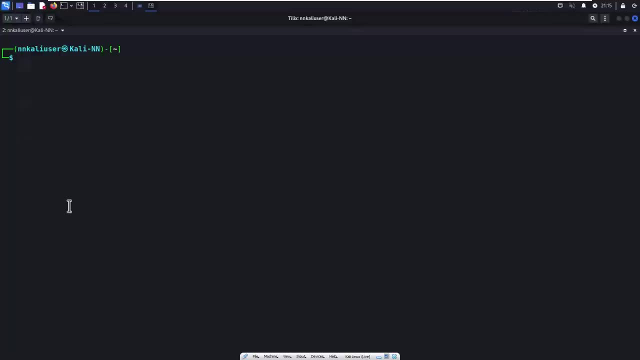 is go ahead and check out the two videos I have in my Kali Linux security tool series, where I cover the first half of Metasploit, which is the initial exploitation phase, how to use it, how to use all the modules and all the great stuff inside it, And then I cover 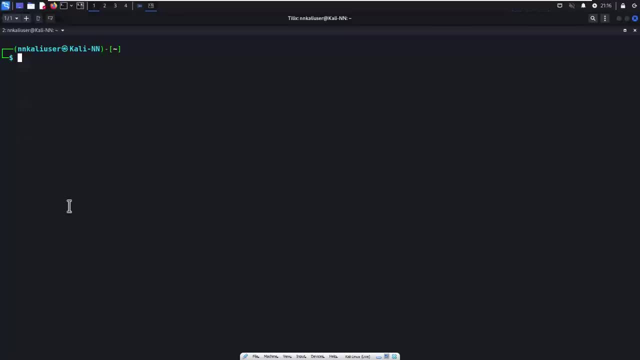 the post exploitation, how to set up persistence, and things like that. So, anyways, I'm going to open up one of the many interfaces of Metasploit, And this interface I'm going to use is called msf-console. Again, really long video here, So forgive me if I sound like I'm rambling here. 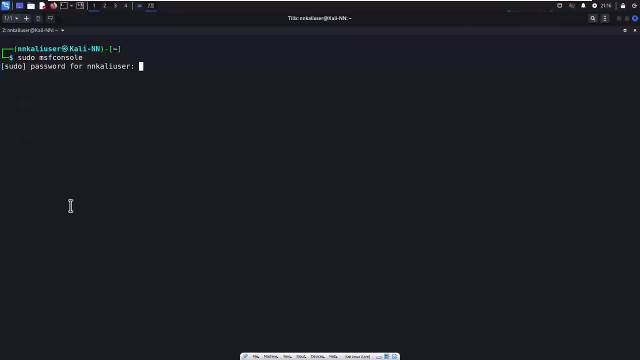 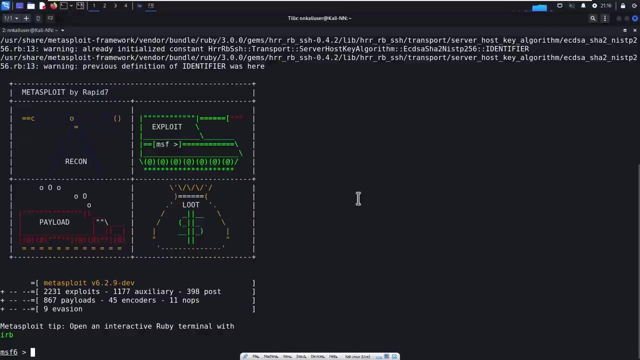 So we're going to do msf-console and we're going to go ahead and let it open up after I give it my password, And it shouldn't take too long- And then we're going to get a bunch of text, And And here we are. So at this point, what we're going to do, we are going to search. 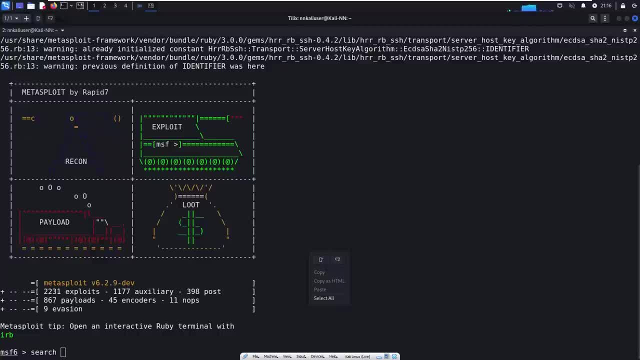 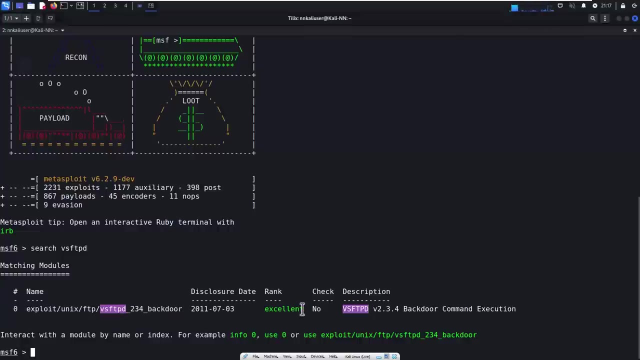 for vulnerability And I thought I had it copied, but apparently not, So I'm going to copy it. right now We're going to search for a vulnerability with that FTP that we saw earlier on that Linux machine. So what we do is we search for vsftp. Here we go. We got a hit. It says it's an excellent. 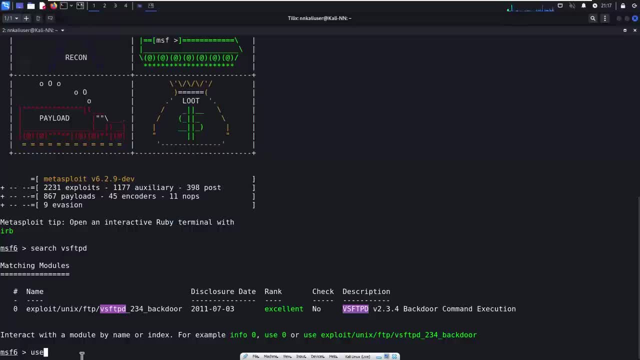 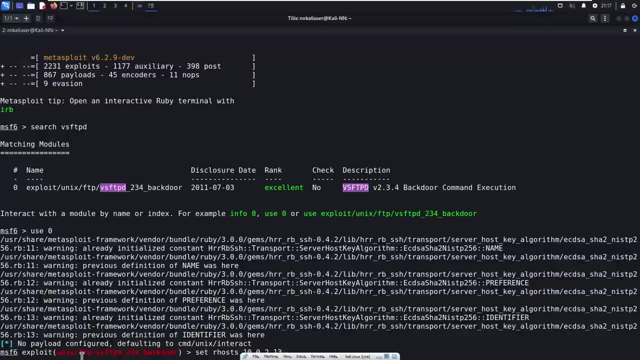 That means it should work, hopefully, And what I'm going to do is I'm going to hit use zero And then I'm going to. I'm going to set my rhost to the IP of that machine, which is 13.. And at this point, all we have to do is 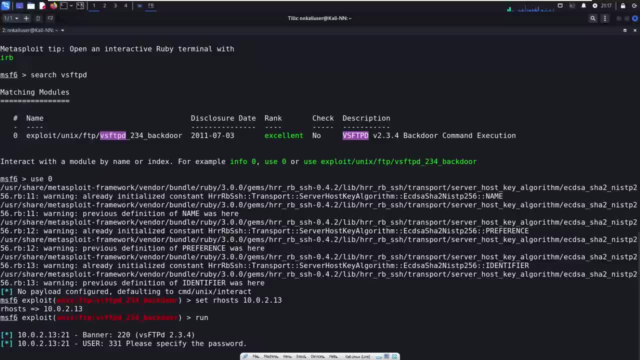 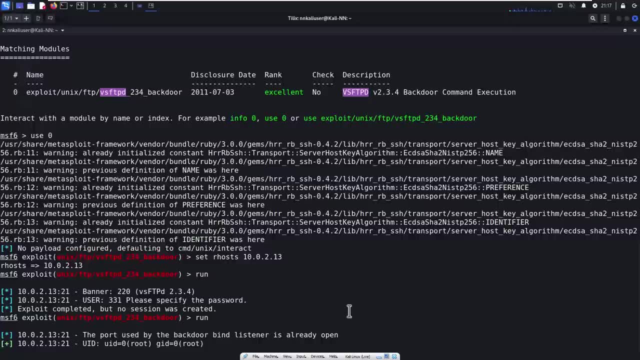 hit run And we're going to have to wait here for a second And it looked like it denied us. Apparently, it didn't want to be nice there, So we're going to do it again because we are persistent. Actually, we'll do persistence later in another video. Actually, check out that second video on. 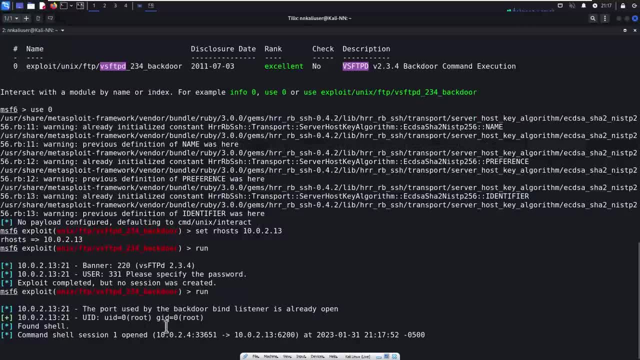 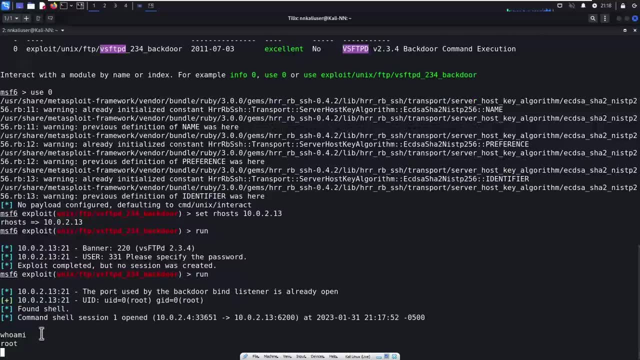 post-exploitation for that. So at this point it looks like it actually worked. I don't know why. we had a little hiccup on the first run, but we're good Second one, And I can prove that by going: who am I? I'm root. Okay, Well, you knew I was root. 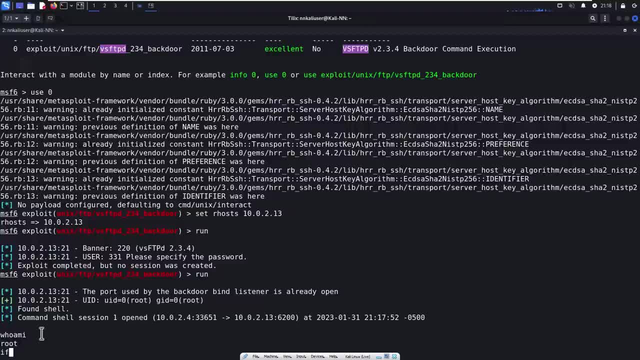 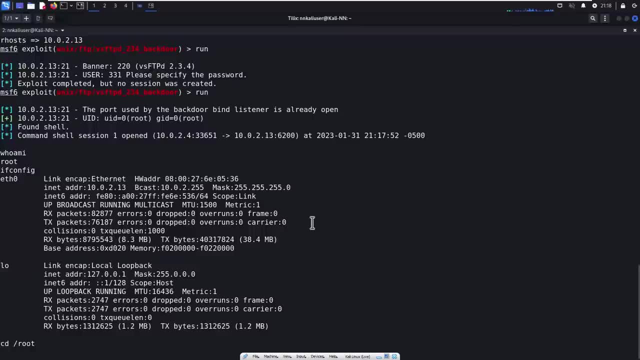 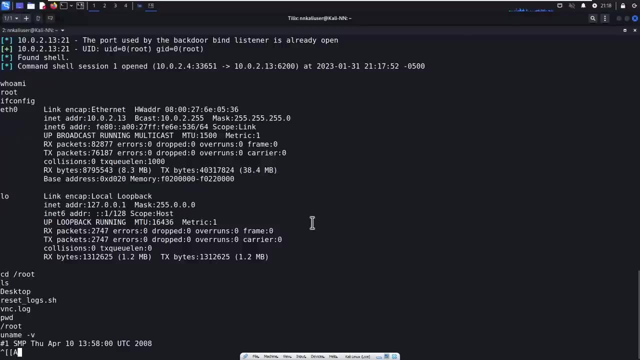 probably I'll log in in here because I did sudo right. But watch this. I'm root on this server And I can prove that I can go here And there I am. Well, that didn't quite work, did it? And there you go. You can see I am not on my Kali Linux box. 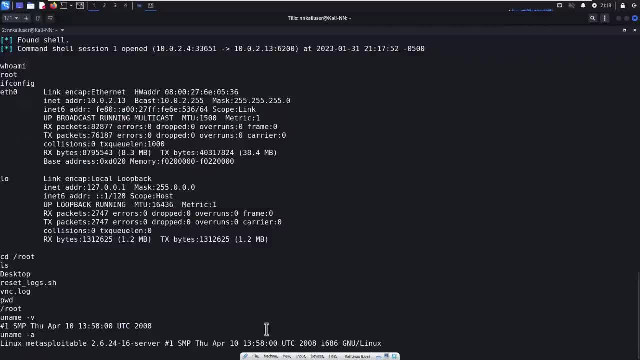 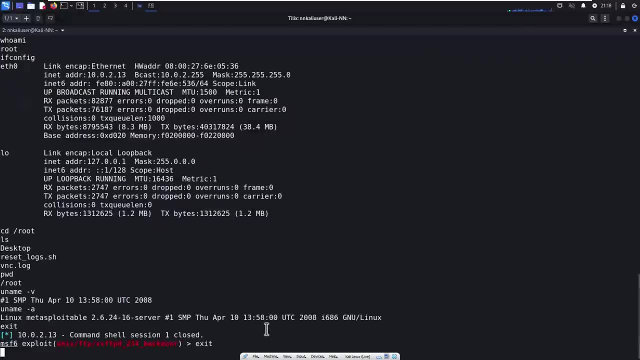 I am on the Metasploitable server, which is ironic because we're using Metasploit to hack a Metasploitable box. So, anyways, you can see that was pretty easy to accomplish, right? So we're about to close it. 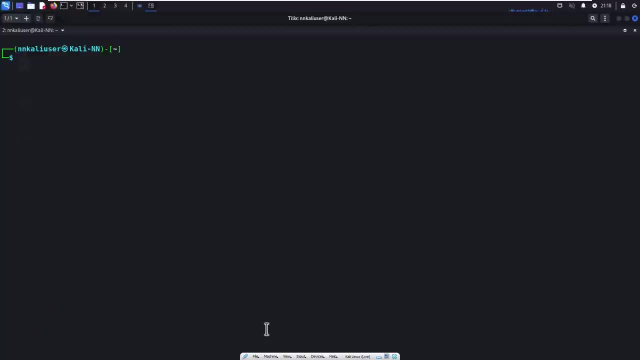 up. But before we do, I mentioned some things you could do for defensive measures as a system administrator. But just to give you some key advice here, and these are things as a pen tester, you would want to offer in that report that you're going to now do that. you've now proven that you. 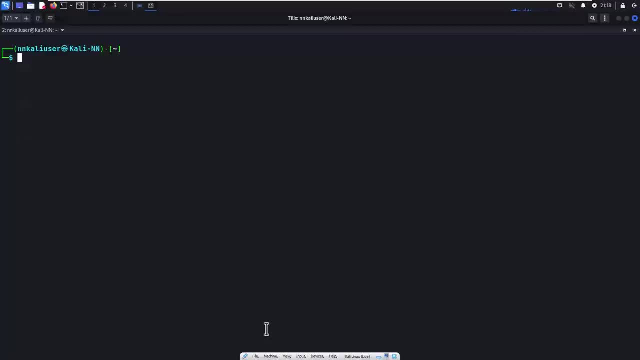 could exploit those vulnerabilities. Some things you're going to suggest: they need to keep their servers patched, And that's not just the server itself. They need to keep the applications and services running on those servers patched. They need to get rid of servers that are past. end of. 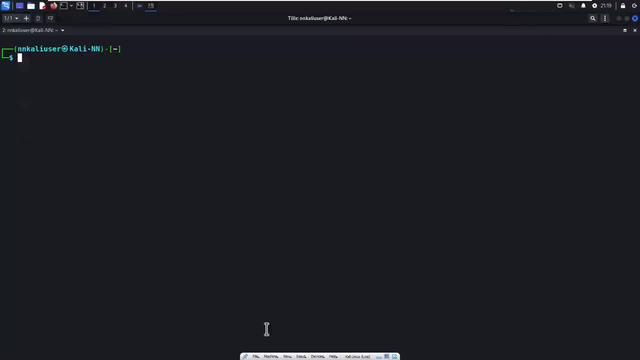 life, Windows 7, Windows XP. why are they on here? They need to check their logs, They need to have good backups, They need to shut off unneeded ports and services, They need to harden those machines And they need to be aware of what is out there. sign up for security feeds, all that great stuff. 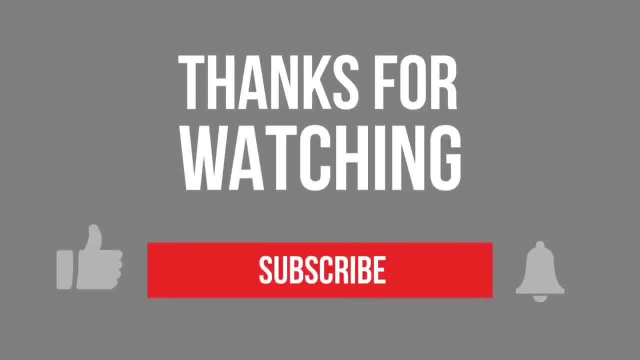 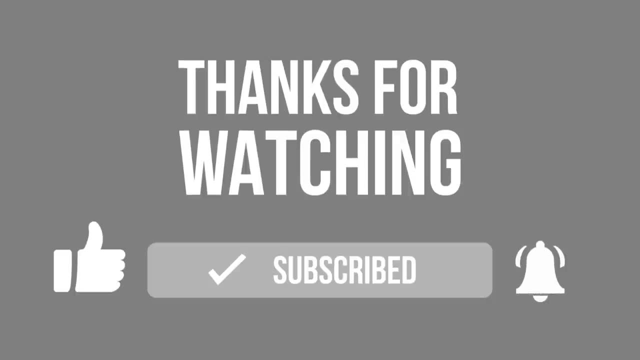 So I hope you enjoyed this video. If you did again, I would greatly appreciate a like. subscribe to the channel for future content. And that's all I have. I'm done. That's all I can handle now. So you have a great rest of your day. Talk to you later.